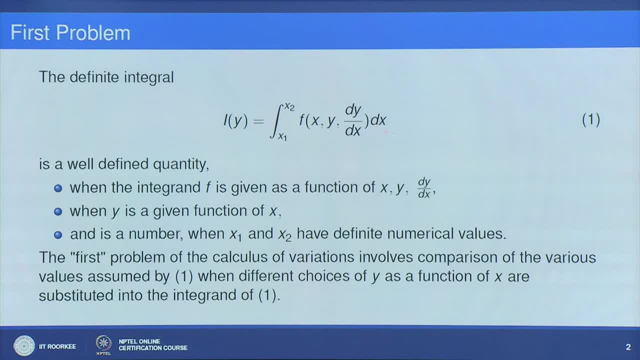 y, d, y by d x, and this integral is with respect to d of x, and we know that this is a well defined quantity, provided that this integrant, f, is a given function of x, y and d, y by d x, and here y is a given function of x and this will give you a number. provided this, 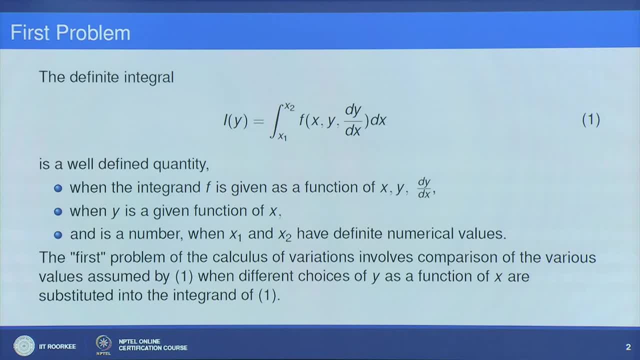 x 1 and x 2 are having some kind of definite numerical value. So we know that that in calculus of variation the first problem ah is to find out, say ah, the values corresponding to different, different functions y, and we compare ah the values of 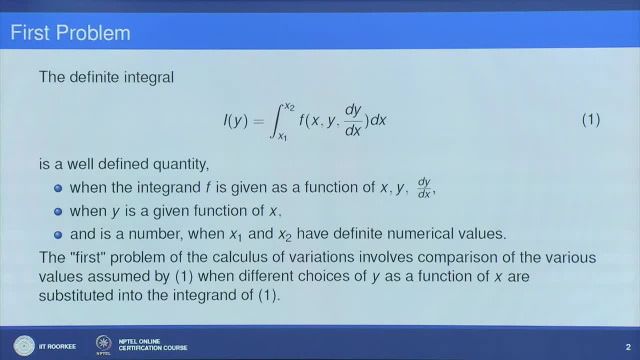 these definite integral corresponding to the given ah, ah function y. So we can say that the first problem of the calculus of variation involves comparison of the various values assumed by this integral, ah, denoted by 1, when different choices of y as a function of x. 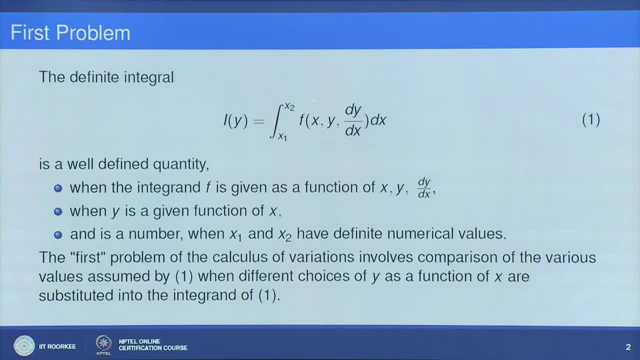 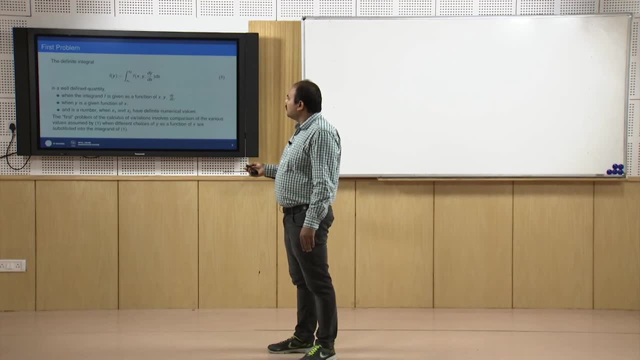 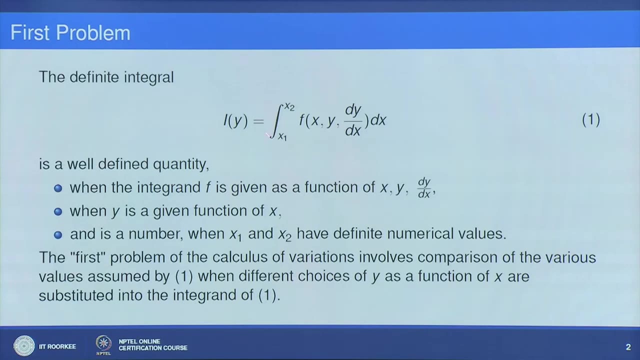 substituted into the integrant of 1. It means that we have a value if y is replaced by some y 1, and then if we replace this y by some other function, say y 2, then we may have two ah different values of this integral and in calculus of variation we try to compare these. 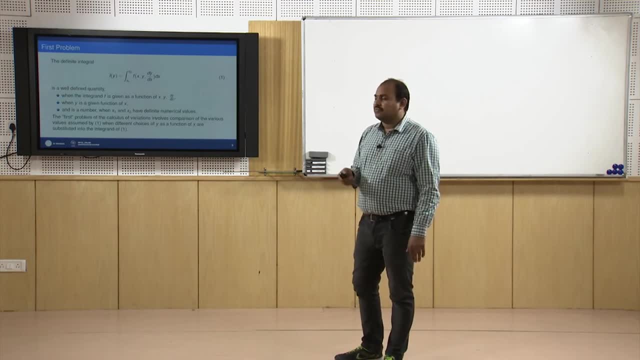 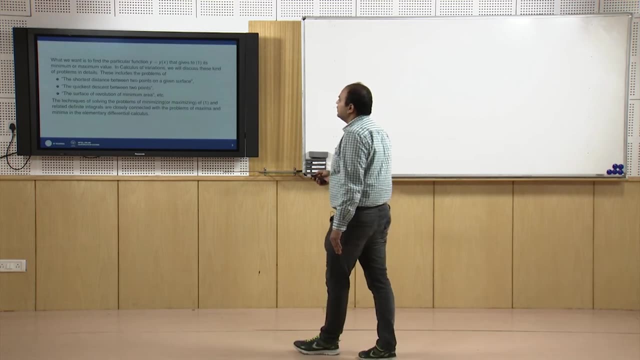 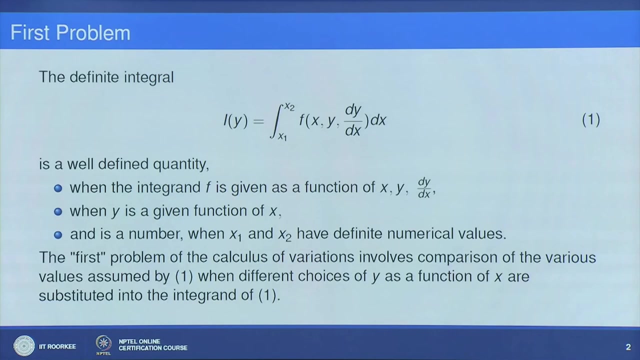 two values and try to find out a function for which the value of this integral is either maximum or say minimum. or you can say that here we want to find out a particular function, y, which is a function of x, that gives the value of this- ah different- integral as its. 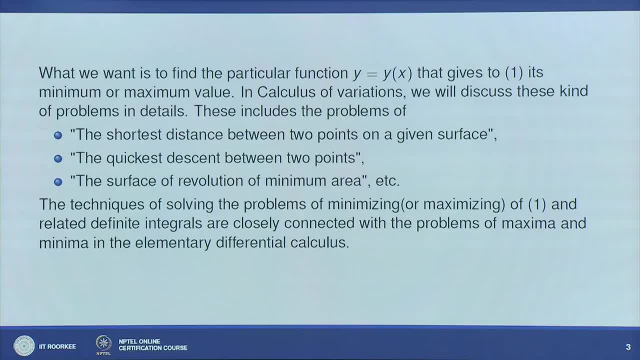 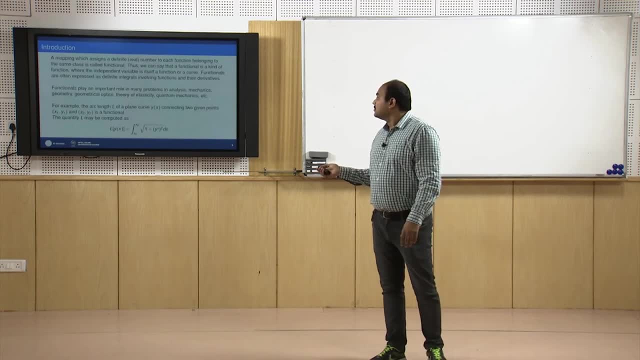 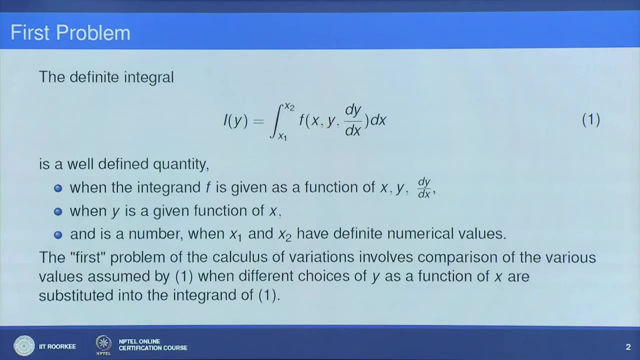 minimum or maximum value. So it means that ah, once ah, ah different integral is defined in terms of ah, say functions of this. another function, y of x, we try to find out, say a function of y in a way such that this will achieve its maximum or minimum value. right. 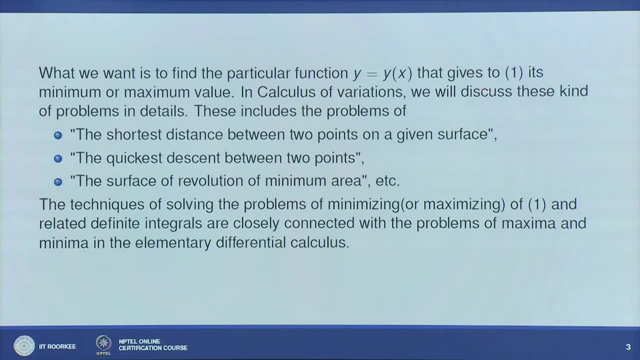 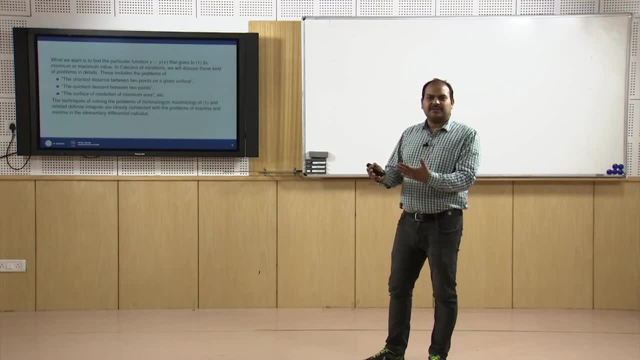 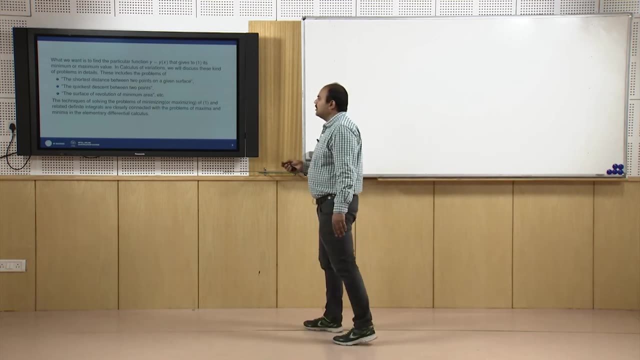 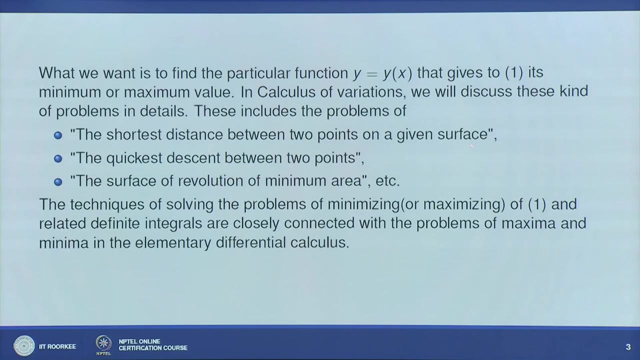 So in calculus of variation we will discuss these kind of problems in details. So in calculus of variation we try to consider problems which can be transferred into this kind of definite integrals. So here there are certain problems, and some problems includes the problems of shortest distance between two points on a given surface, What it means. that suppose 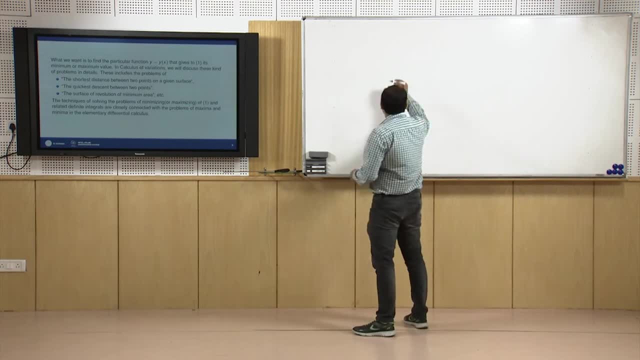 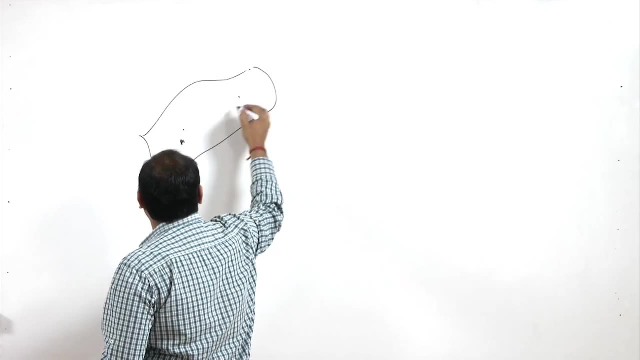 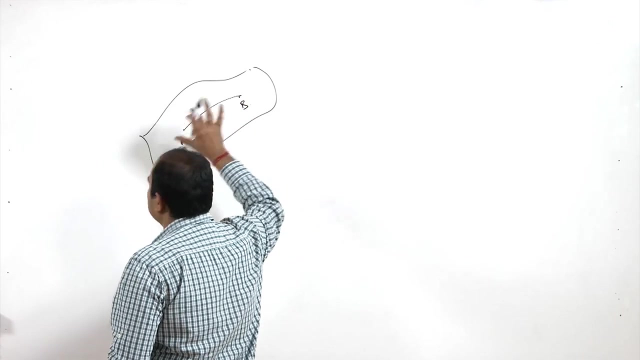 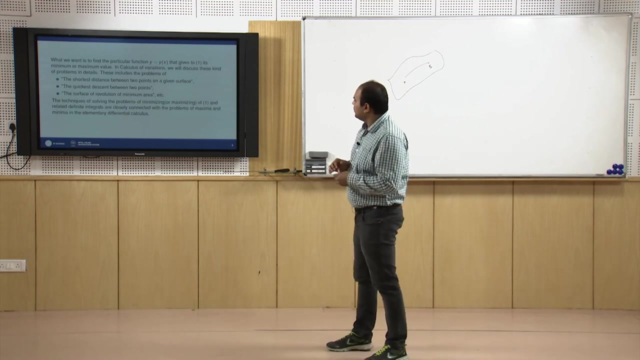 we have a surface. it is like you have a surface here and then you try to find out that there are two point, A and B, and then we try to see that what is the shortest Distance between these two point, provided that these two points lie on a given surface. So this is one of the problem discussed in 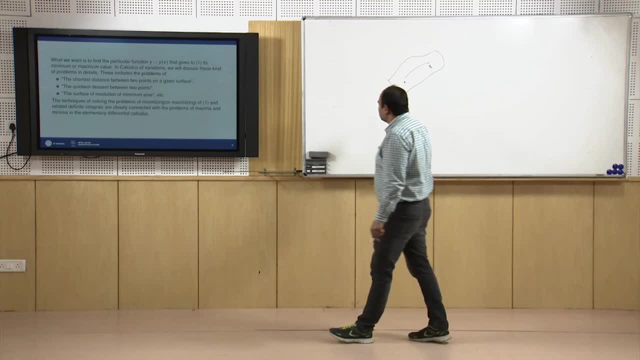 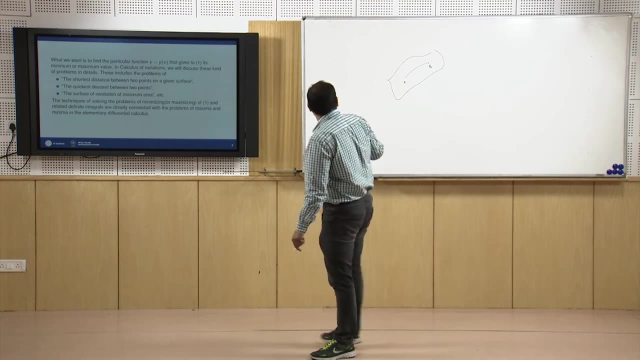 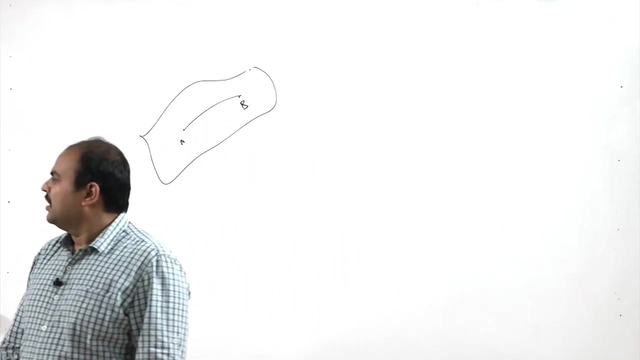 calculus of variation and we will discuss this problem in detail as the problems known by geodesics. So such curves, which gives the shortest distance between A and B, are known as geodesics that we will discuss in due course of time, and the 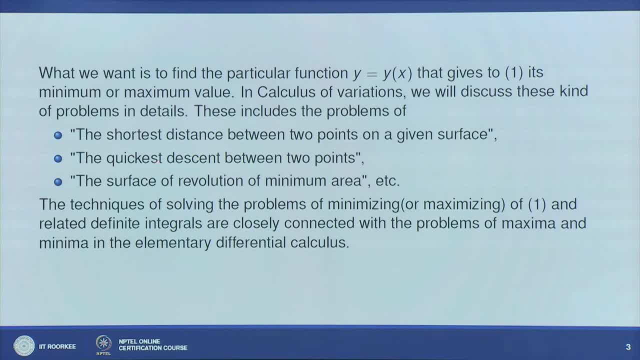 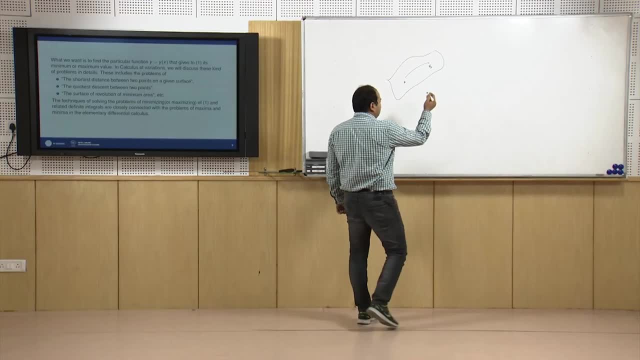 Second problem, very important problem, is the quickest descent between two points. So it means that how we can say: consider this problem, that suppose in a vertical plane we have two point, A and B- of course they are not on a same height, and then we try to find: 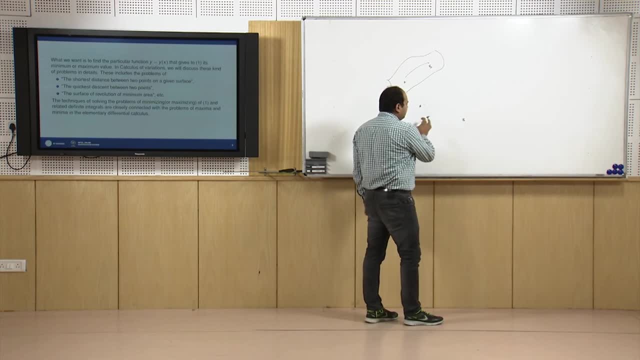 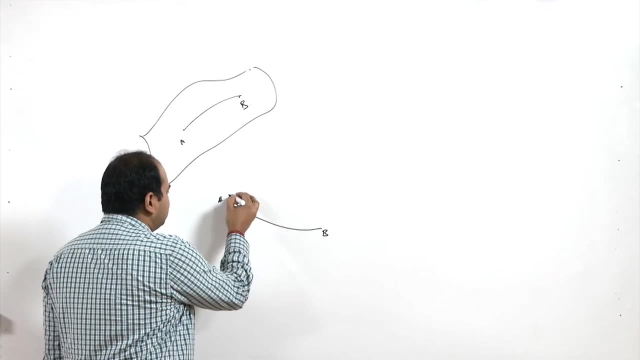 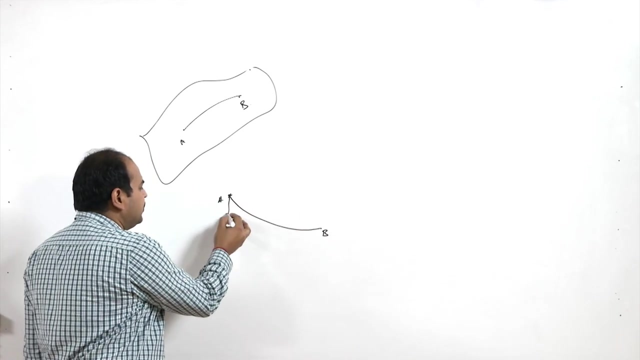 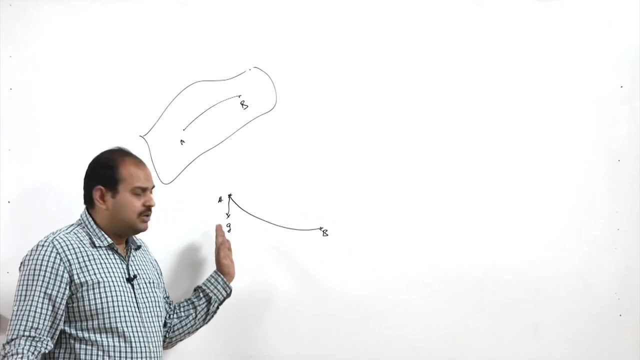 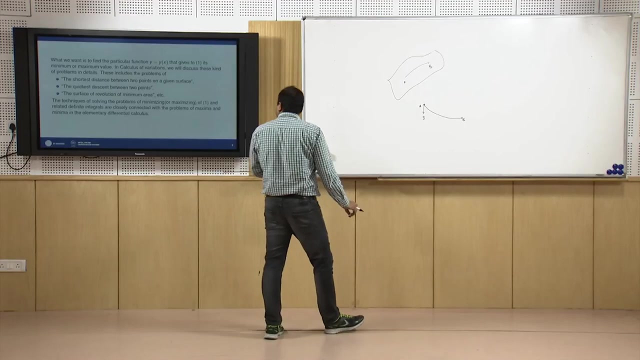 out the curve connecting these two point, A and B, in a way such that the if we take any particle, Say, which start from the point A and it falls under the influence of, say, gravity from A to B, then it will take least time from reaching A to B. So it means that the problem of quickest 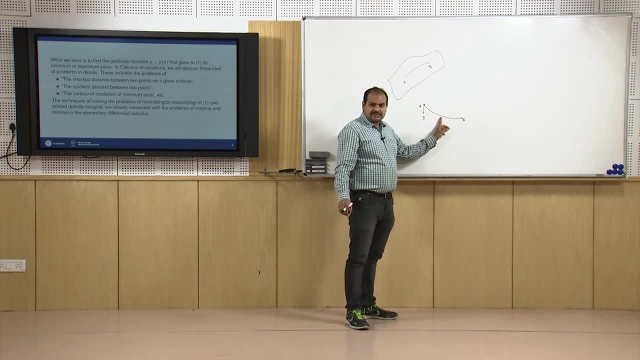 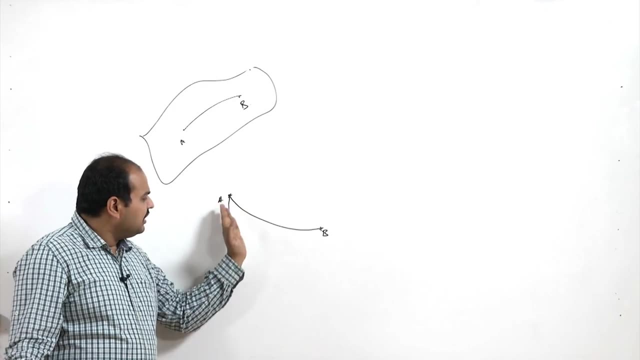 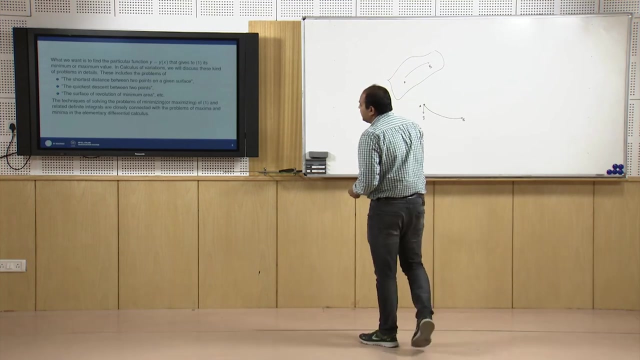 descent is the problem of finding the curves such that under which, if we particle is slightly ста nos- just one frontical will take any time from reaching A to B. the Besides, from A to B under the influence of gravity will take the least time. So that also we will discuss in detailed, and that is the problem known as Bracito Chroma. 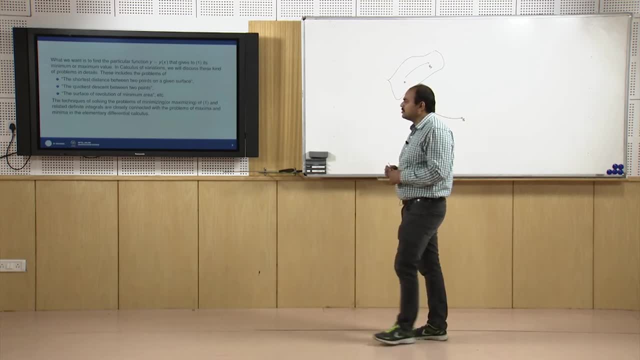 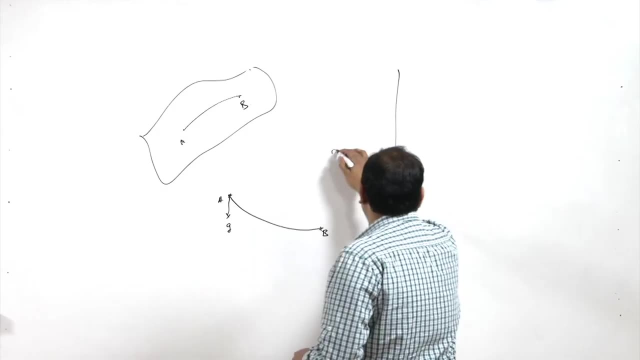 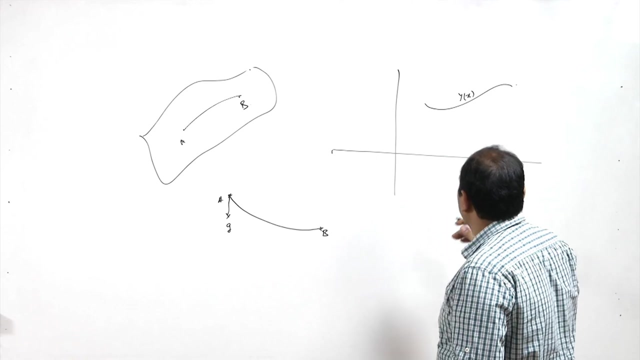 problem- And this is the first problem which is suppose to be the beginning of Calculus of Variation, we will discuss this problem also, and the one more important problem leaders. variation is the surface of revolution of minimum area. it means that ah- suppose we have a ah say, say one function, say a y which is a given function of y of x, then we try to. 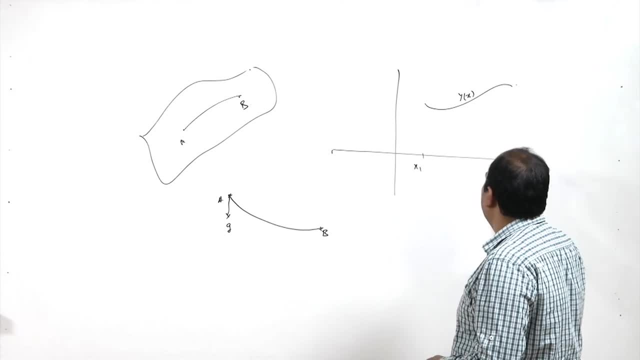 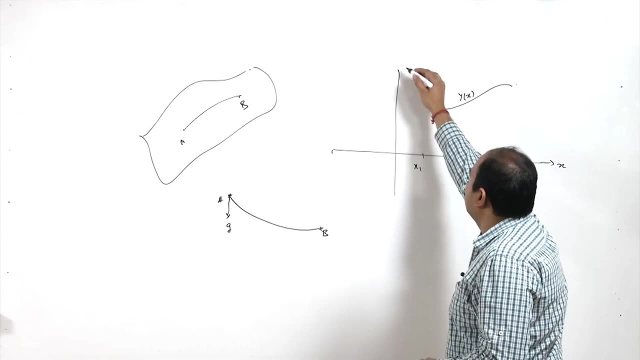 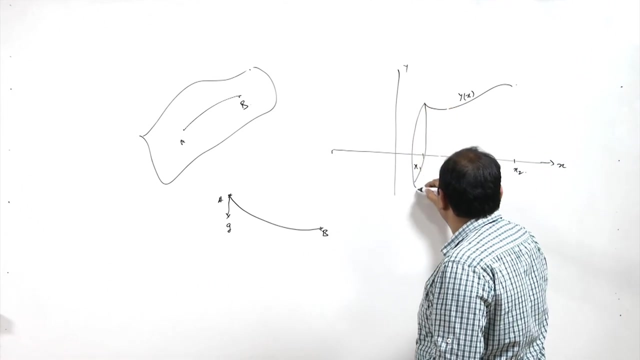 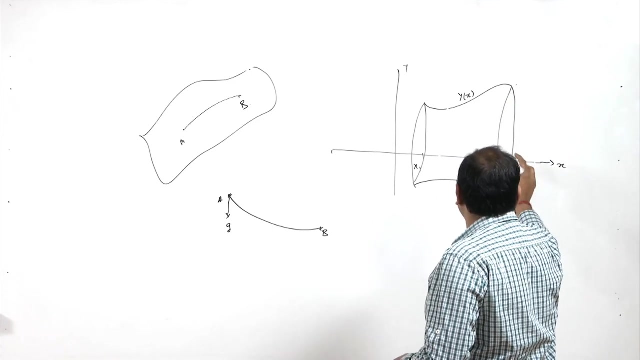 between, say 2 point, say x 1 and x 2. and then what we try to do here? we simply revolve this curve around this x axis, ah, with the angle 2 pi. then it will generate a kind of right ah here, just like this. ok, So here it is x 2, and then we try to check the surface area. 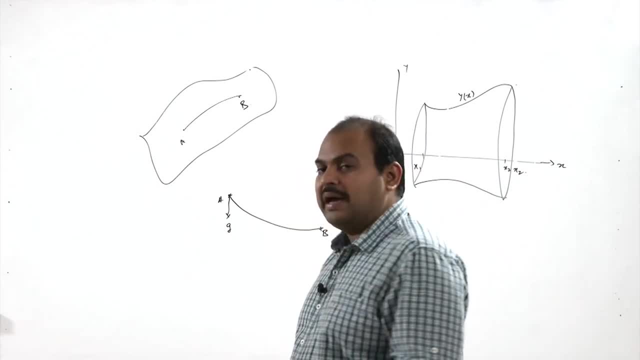 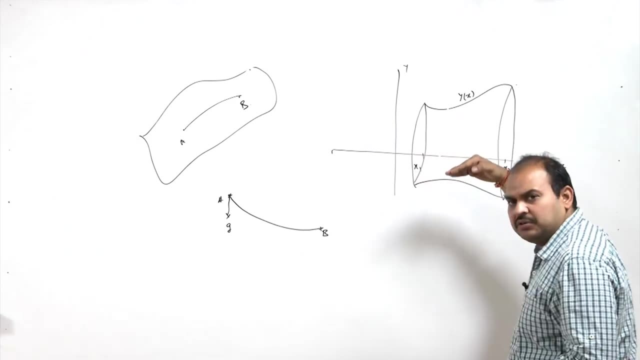 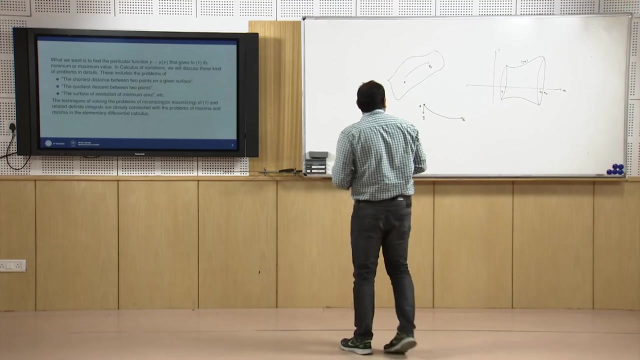 of the ah revolving surface and we try to find out the curve y of x such that the surface area of the figure so obtained has a least ah surface area that we try to discuss in this. So here we try to see that we will discuss. 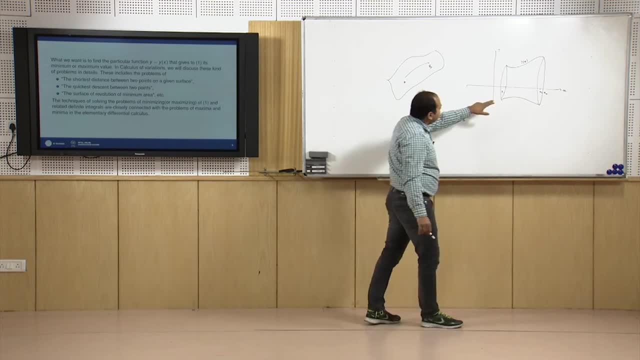 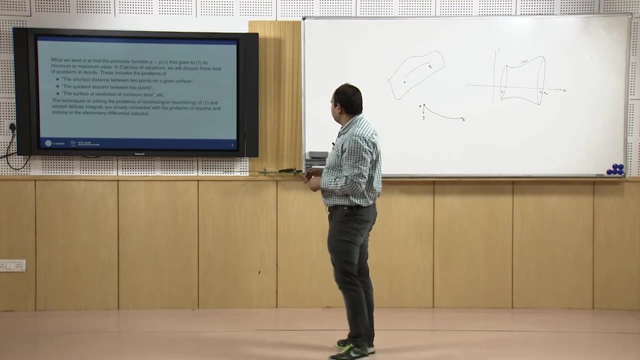 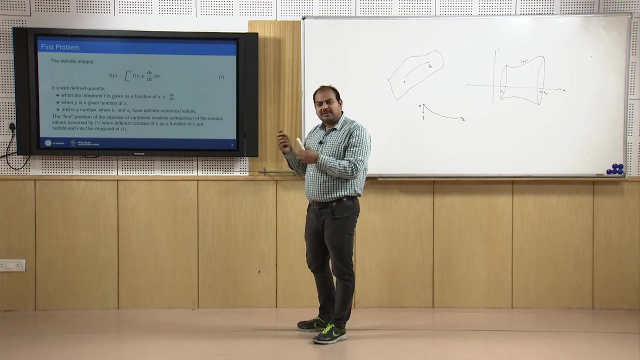 ah, these problem in detail, that all these problems, ah can be reduced. ah in finding the maximum minima of the ah, diff definite integral post like this one. So all these problems can be termed as or can be written in terms of, ah, some kind of definite integral which depend on the ah. ah say some function. 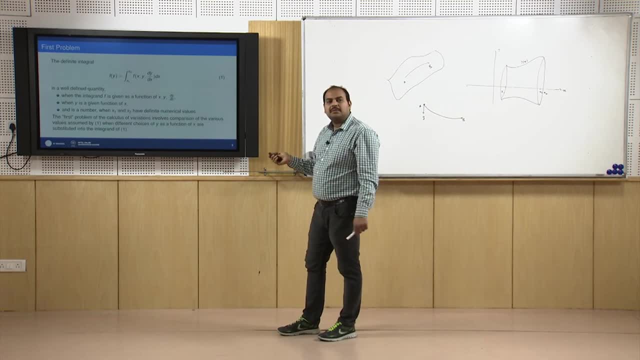 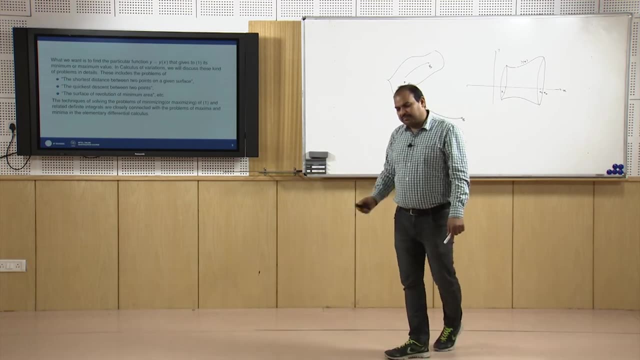 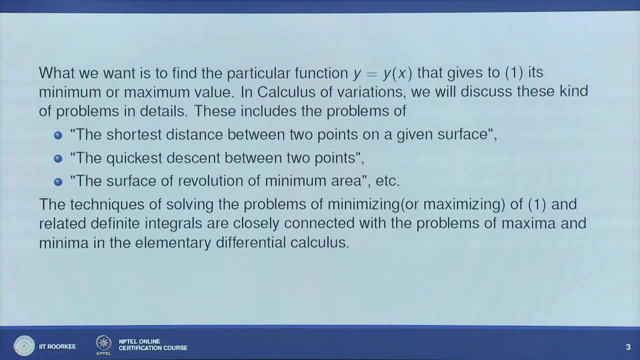 y and we try to find out, say, minimum and maximum value of these different integrals. And these details or these methodology is closely related to the problem of maximum and minima in the elementary differential calculus, or I can say that the techniques of solving the problems of 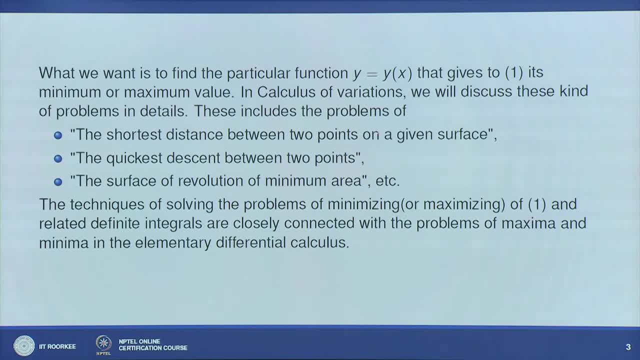 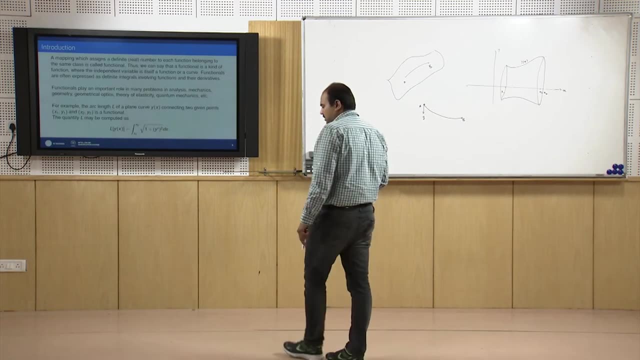 minimizing or maximizing of different ah definite integral given in one and related definite integrals are closely connected with the problems of maxima and minima in the elementary differential calculus. we try to see how it is this. So now, ah, these ah definite integral are: 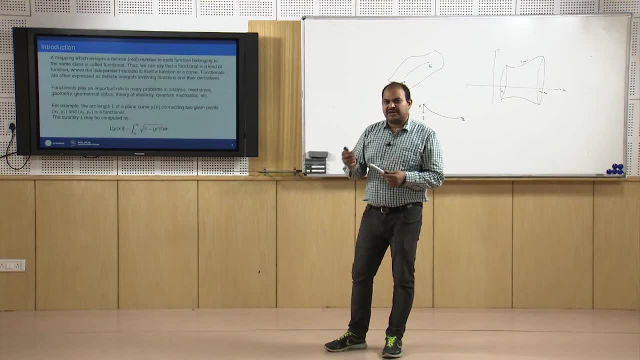 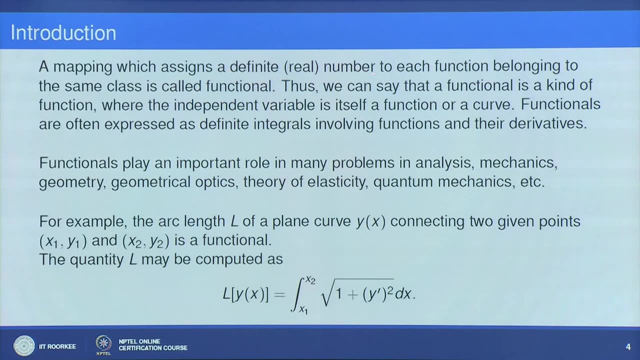 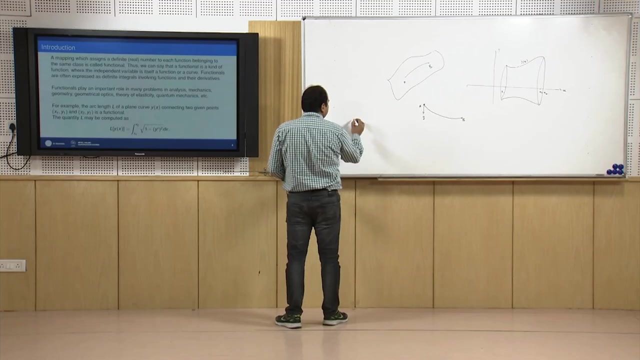 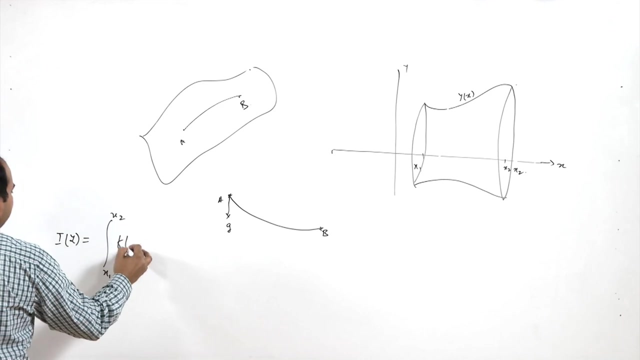 termed as a name which is known as functional. So what is functional? a functional is a mapping which assign a definite number to each functions belonging to the same class is called functional. So if you so, if remember, we have written down our ah difference integral like this: it is from x 1 to x 2, f, x, y and y dash. 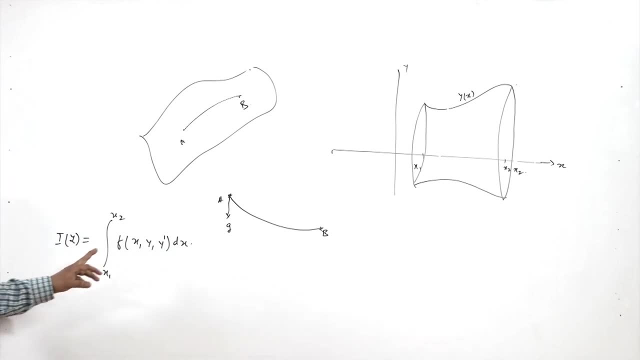 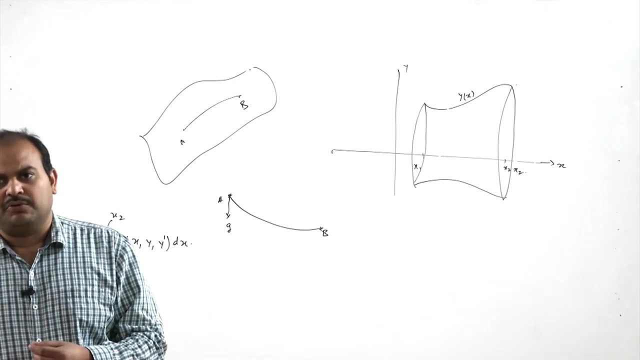 d of x. So it means that if you take a value y here, then the corresponding ah value, ah, is given by I of y. is this? So it means that for any given function y, there is a value given by I of y. So basically it is a kind of a correspondence between a function to a value. 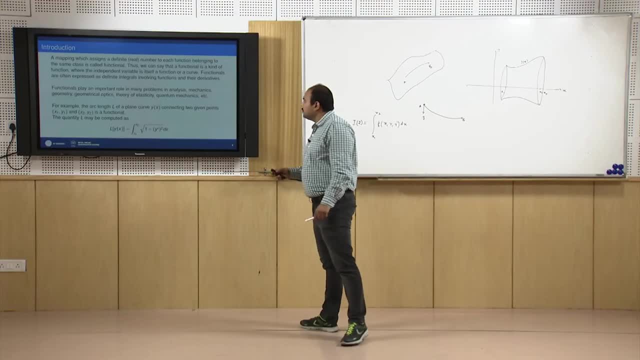 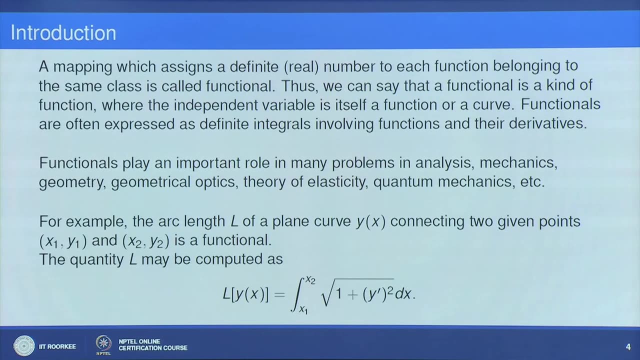 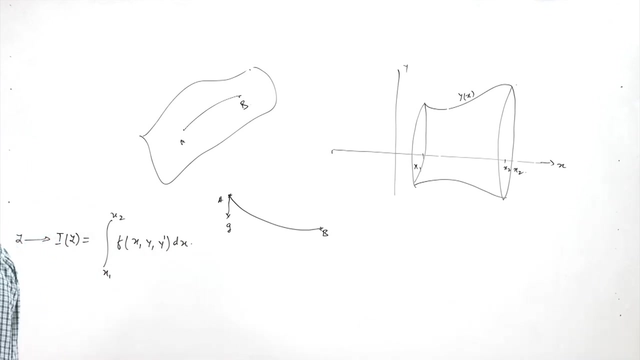 So it means that it is some kind of a generalization of a usual function. So we can say that a functional is a kind of function. So it is a kind of function which, say, correspond between y to I of y. So here we can say that a functional is a kind of function. 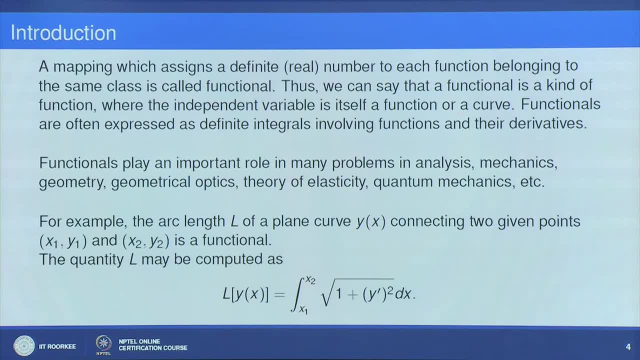 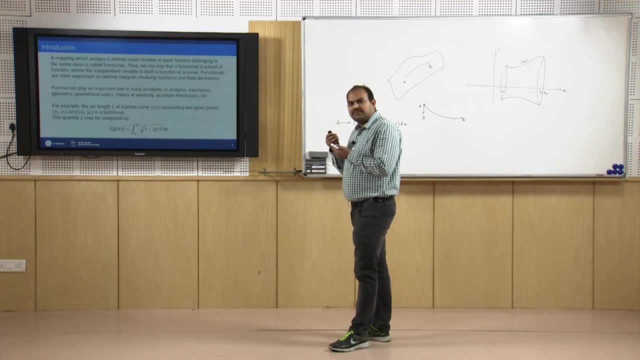 where the independent variable is itself a function or a given curve. So here functional can be generalized as a generalized version of a function. So it is also a functional. the only thing is, that independent variable is already a function of some function of x, So functionals. 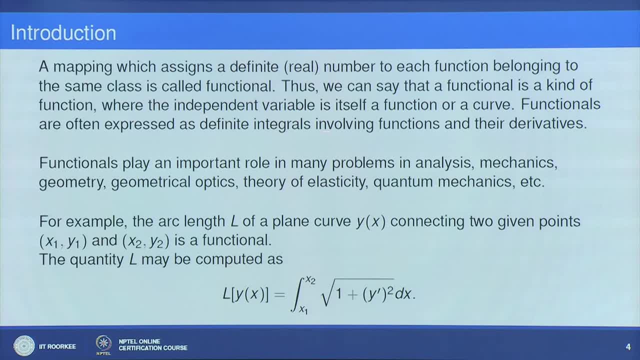 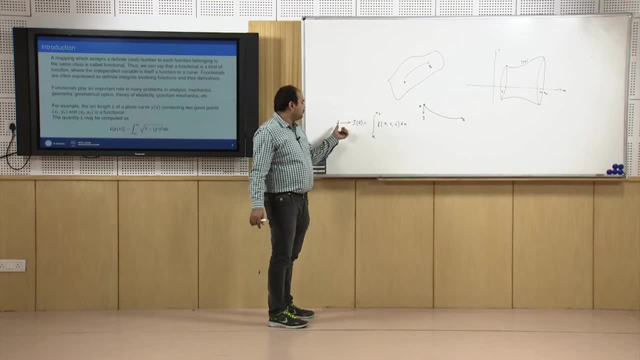 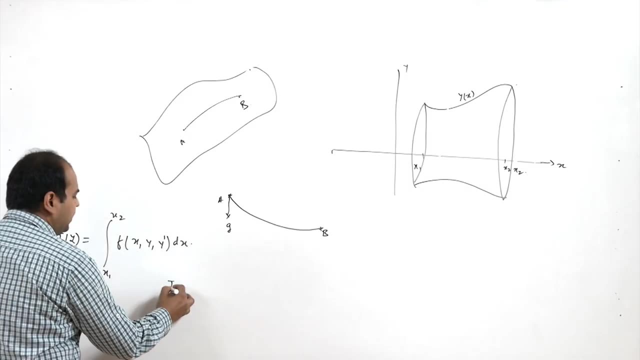 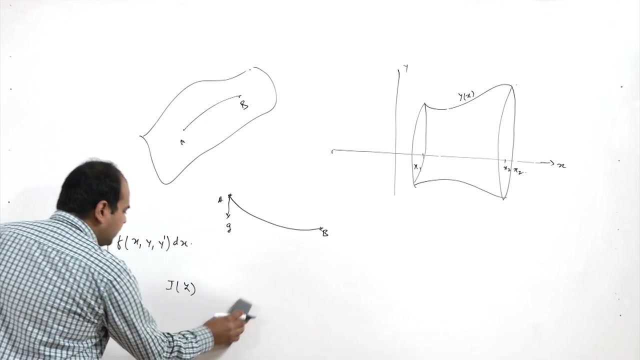 are all often expressed as definite integrals involving functions and their derivatives. So, in general, you can define any correspondence between a functions y to the value I of y, and so there are certain way you can define I of y as say. this will go to say you can simply say you: 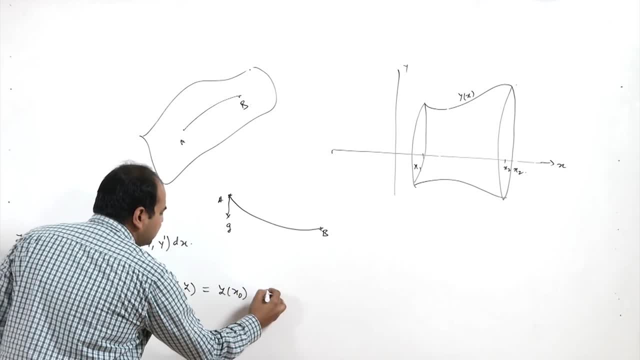 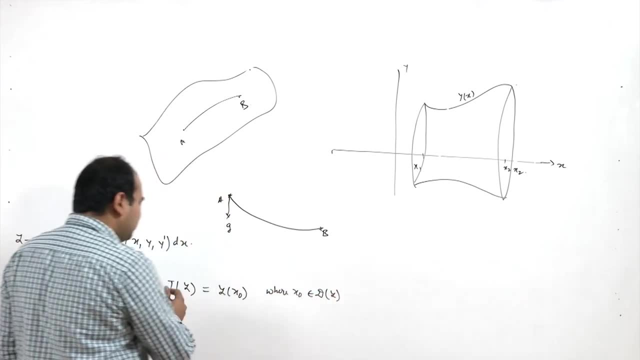 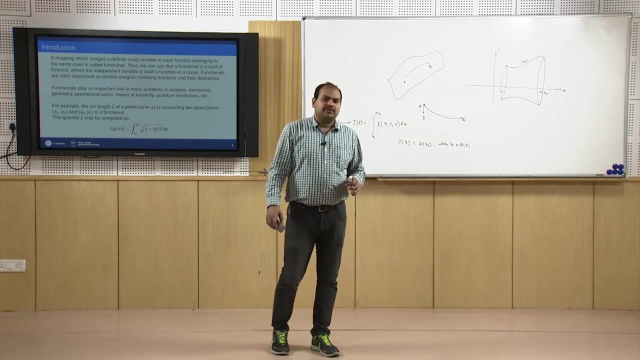 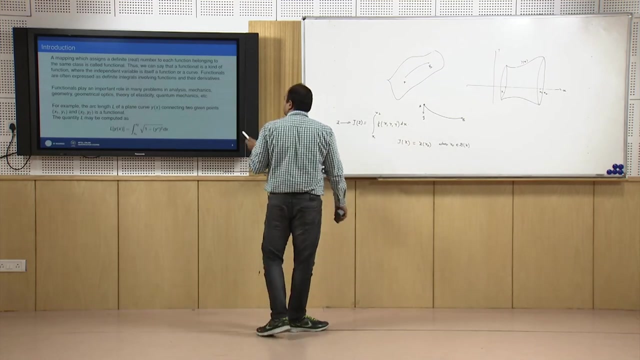 may define it like this also: y of x naught, where x naught is some point in domain of say y. So here also this also represent your functional. but here in calculus of variation we try to consider the functional which are termed as, or which can be written as, these kind of forms. So here we will discuss that functional are. 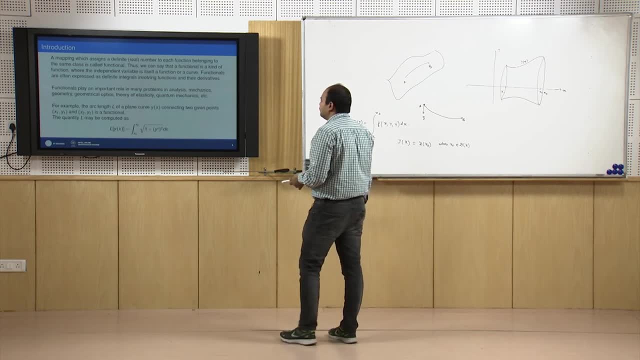 often expressed as definite integrals involving functions and their derivatives. So, in general, we try not to discuss this, So I hope that this is not a very important topic for today's discussion. So thank you very much. Thank you very much. 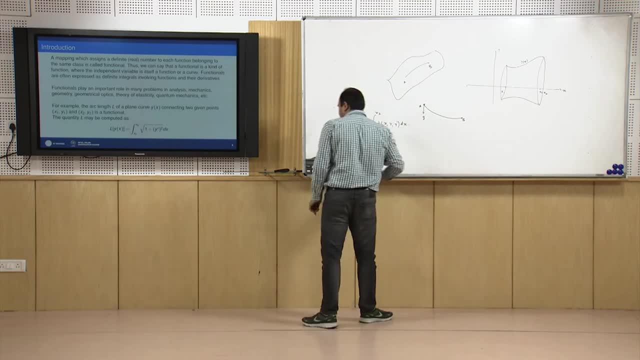 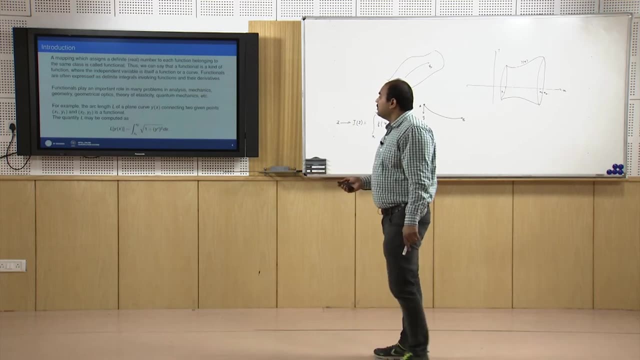 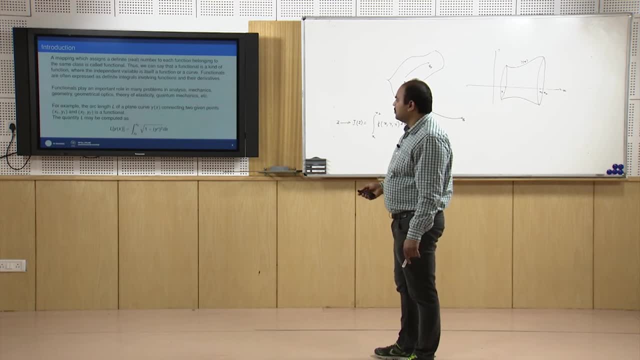 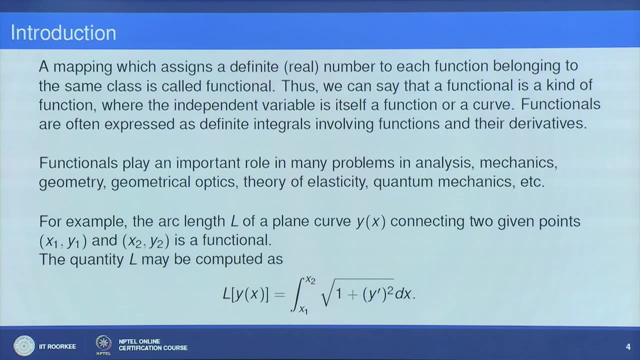 in many problems since analysis mechanics, geometry, geometrical optics, theory of elasticity, quantum mechanics, etc. So that we see as an application of calculus of variation. We will consider certain problems of these fields as a application of calculus of variation. 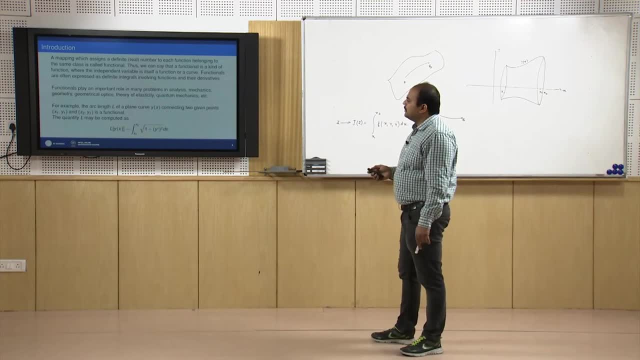 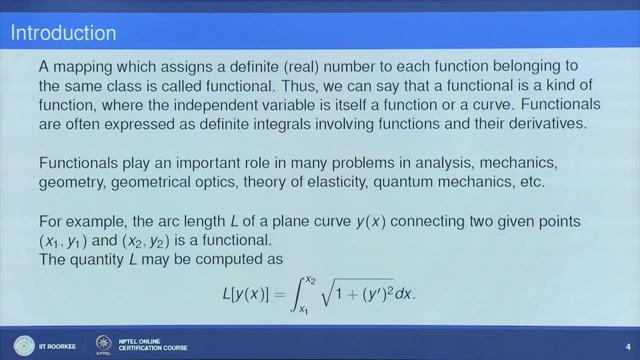 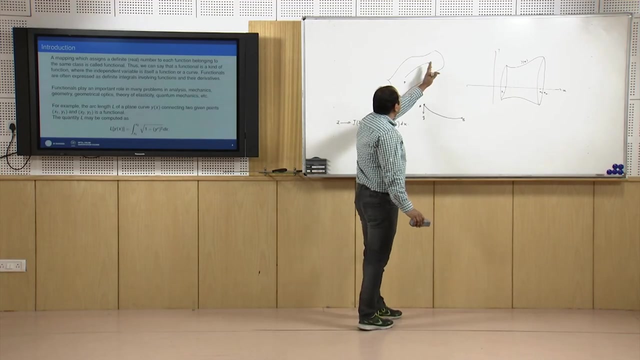 That will shortly, we will discuss. For the beginning, we can say that the arc length L of a plane curve connecting 2 given points is also a functional. What is this So initially, if you remember, if we have a surface and we have a, 2 points, A and B, and try to find out, 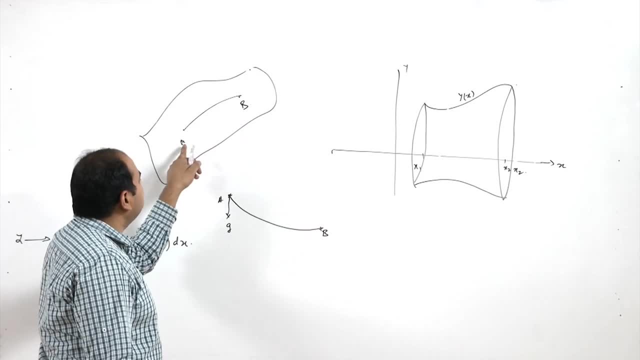 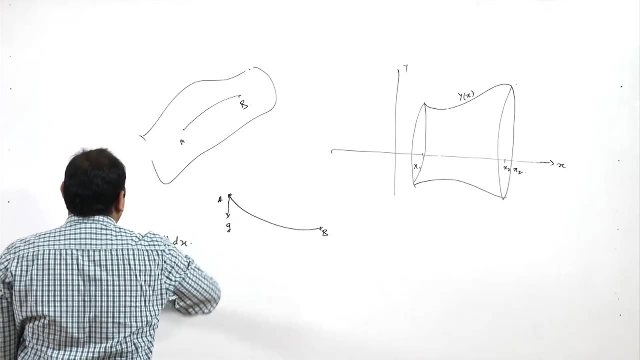 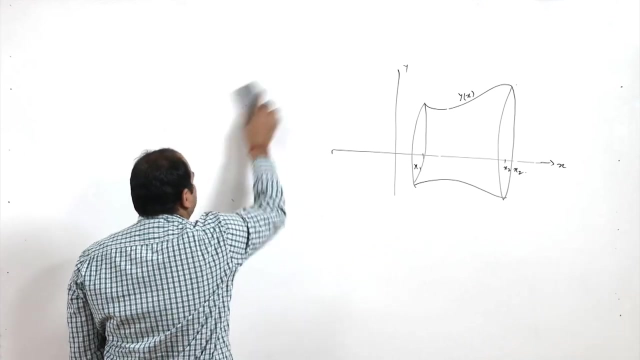 say minimum length, length between minimum length of this curve connecting these two point A and B. So let us say that this surface is a planar surface, or you can say that these two points lie on a say xy plane or yz plane or something like that, and we try to find out. say, minimum distance. 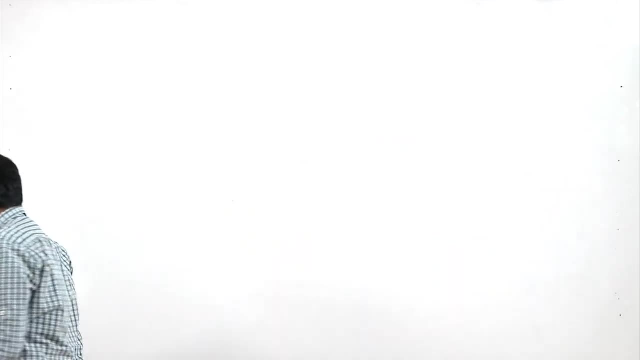 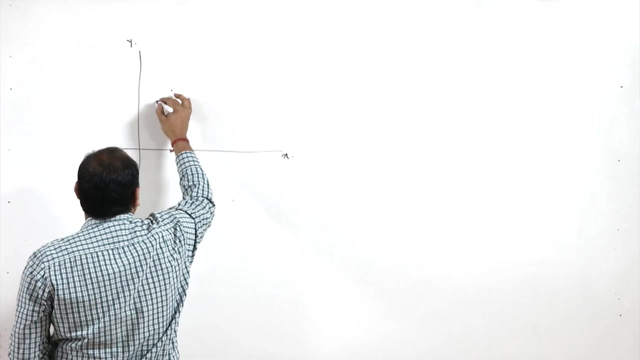 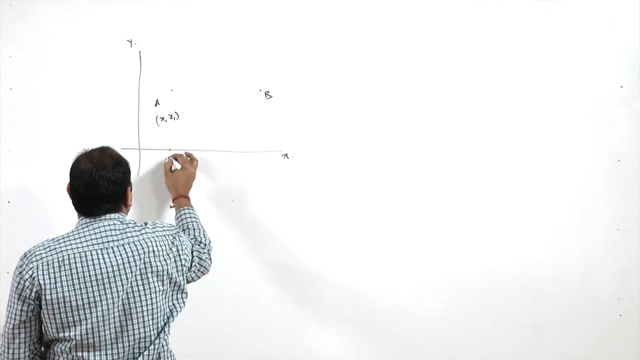 of the curve. So here what we have, let us say that we have a xy plane. So here we have xy plane. and then we have a point A and we have a point B. A is given as x1, y1. So here, this is your x1 and the corresponding is your y1. and here 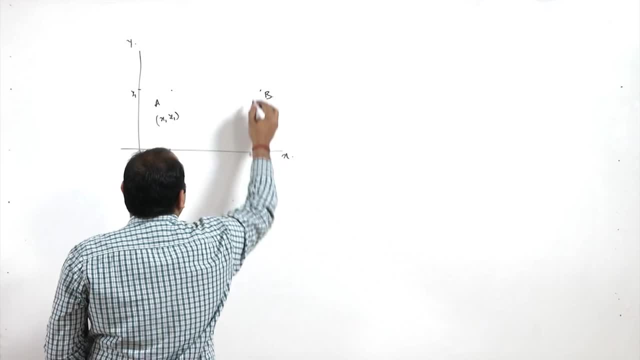 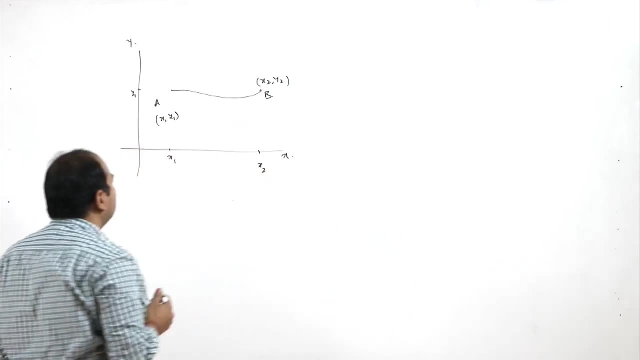 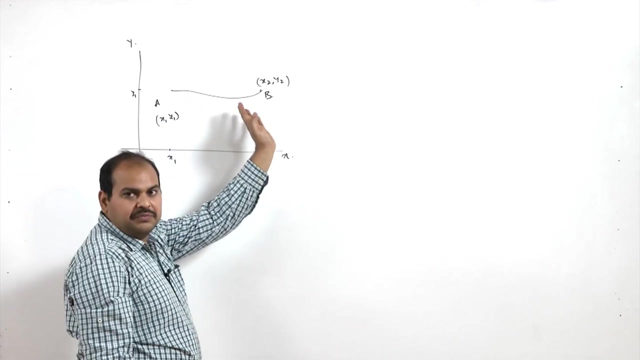 we have say another point, say x2, y2.. So here we have x2, y2 and then we try to find the. we can draws many curves connecting this A and B And we try to find out that curve which minimizes the length of the curve connecting this A. 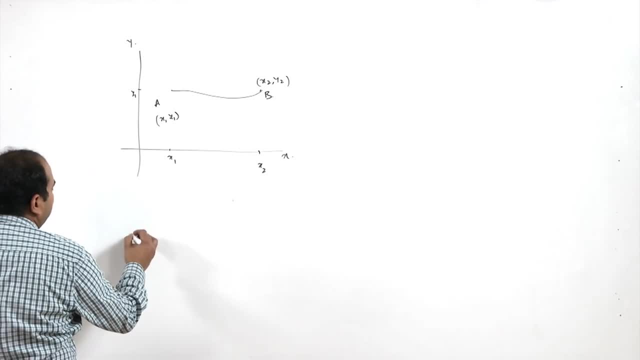 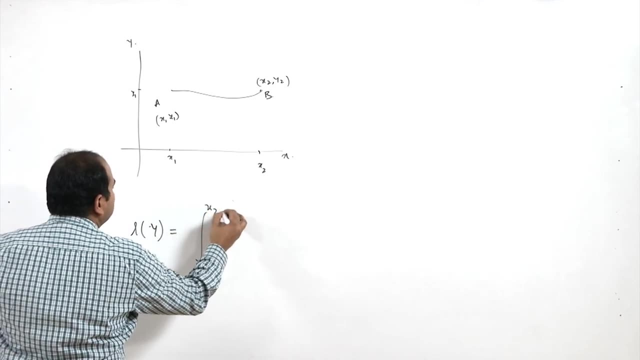 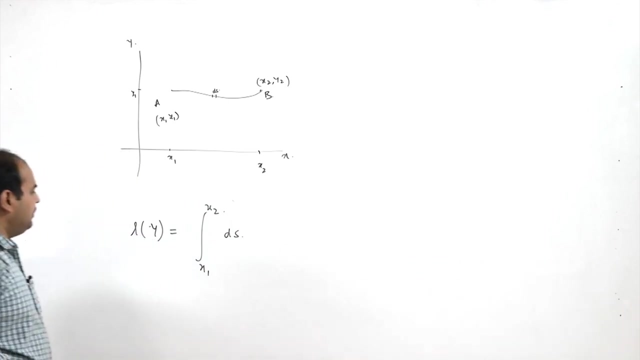 and B. So here I can say that if we look at the length of y, it is given by say x1 and x2, and if we take this as d of s, then we can simply write d of s. So it means that 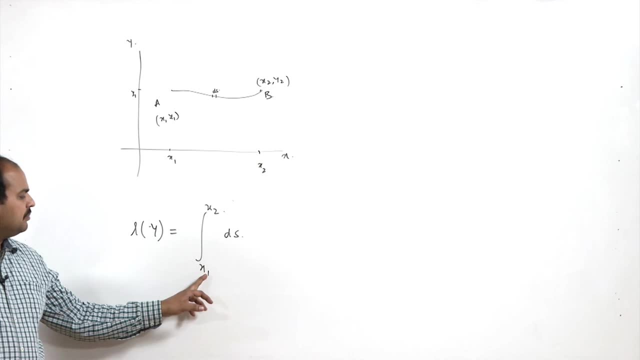 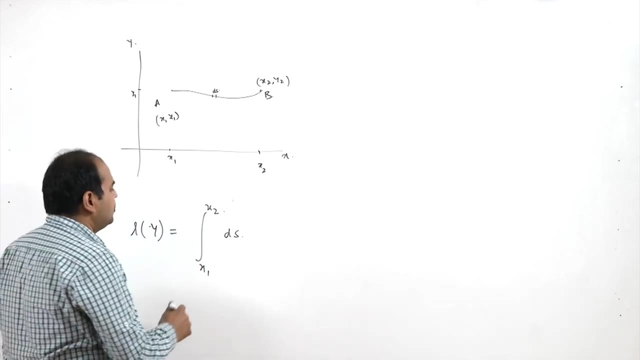 length of y you can define as the integral between x1 and x2.. So colour. so when you learn you have to sample like this: and then those you should write along this line and the mates on the point A, where x1 and x2, we know that x1 is. 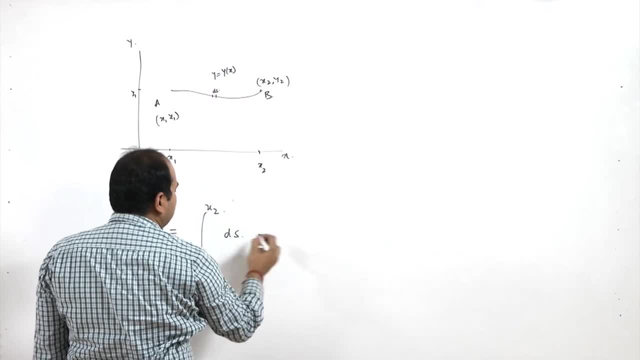 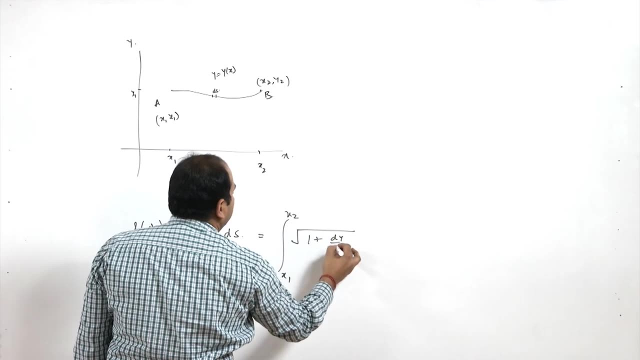 the link that we are choosing between x2, which also gives us the learning painting for line A, And, in other words, if you represent the 이미 chagrin of x class and the executed Back, Deus killed on X, and these will help, you would rather understand the 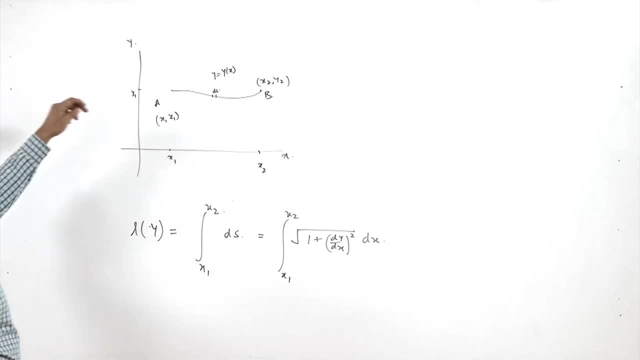 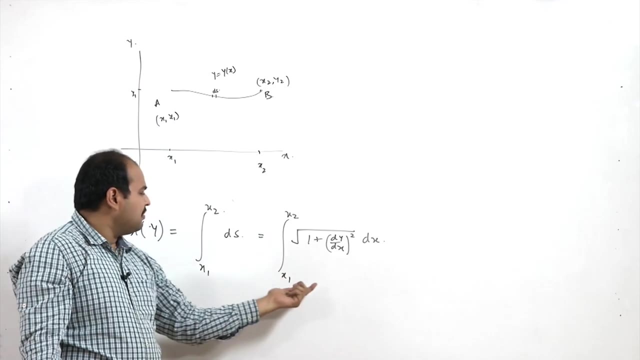 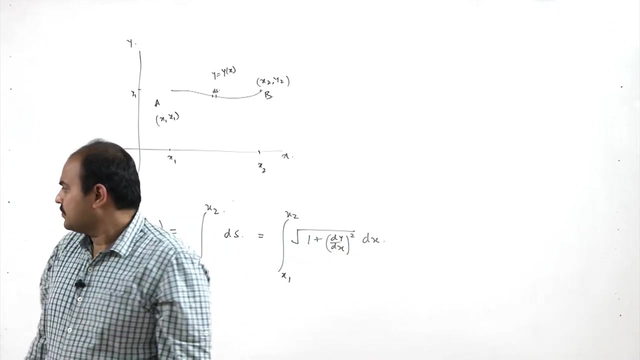 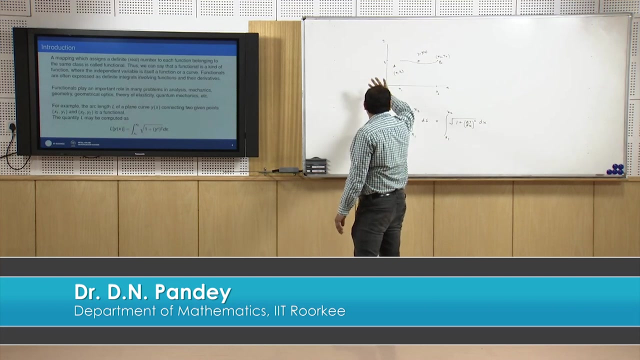 So we can say that the length of the curve connecting A and B is given by this functional, and this can be simplified into this: x1 to x2 under root, 1 plus dy by dx, whole square d of x, and then this is one of the functional we are discussing Now in case of planar region. 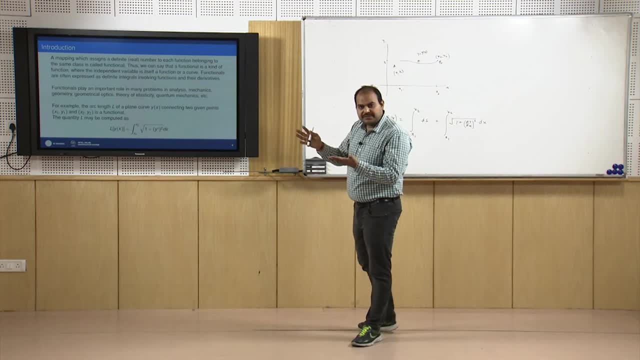 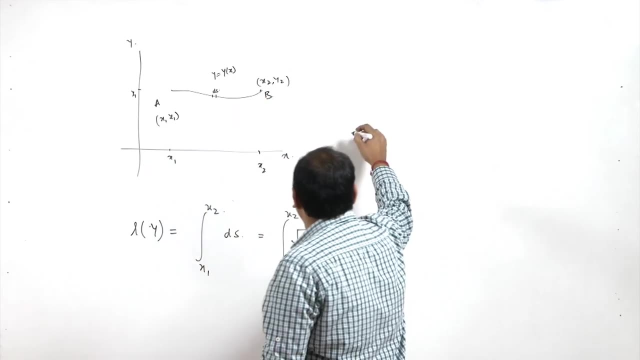 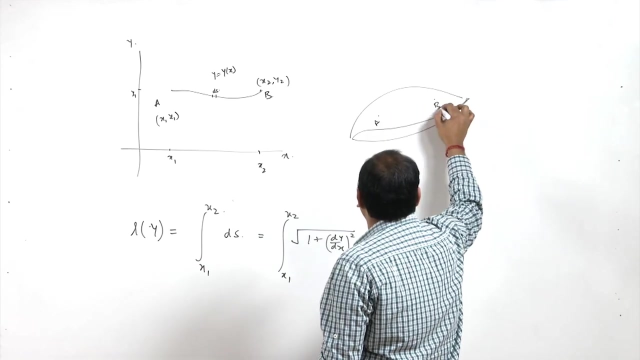 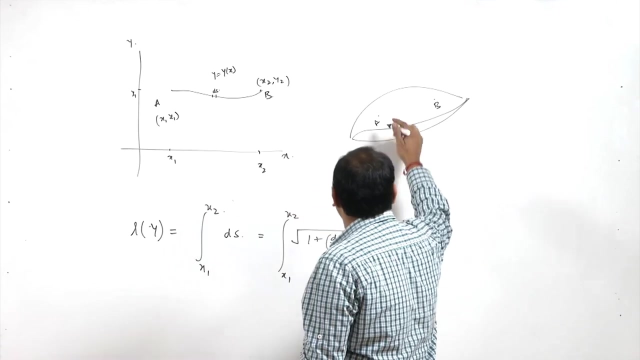 if we consider these two points lying on a surface, then it means that, in place of A and B lying in a plane, if we say that it is lying on some kind of- say, some kind of a surface, then not only we have to minimize the or we have to consider the length of y, but also we have 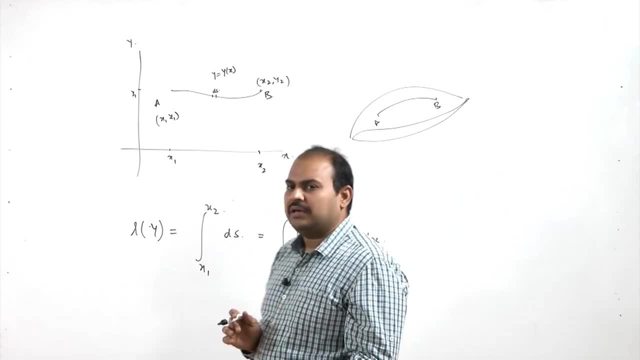 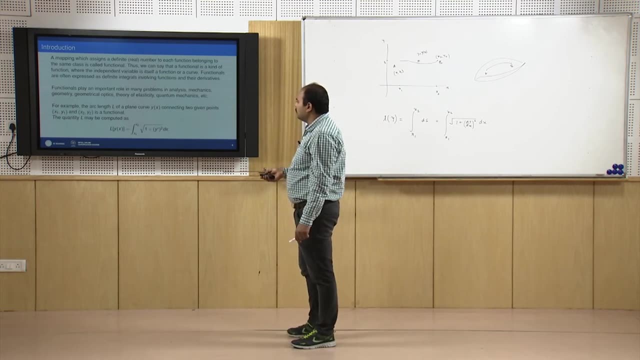 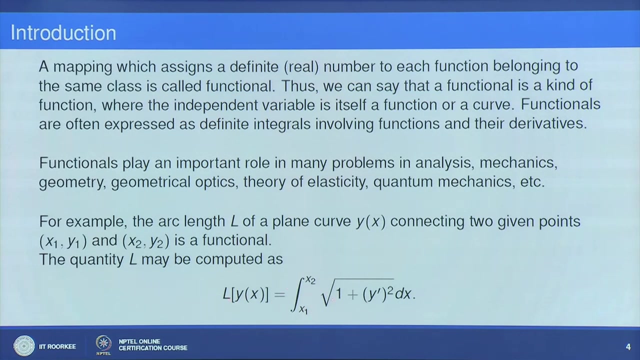 to put a restriction that these two point, A and B, lying on a given plane. So the length of a curve connecting two points is termed as a functional here. So here we can say that this L y, x is given in x1 to x2 under root 1 plus y, dash square d of x. So here if 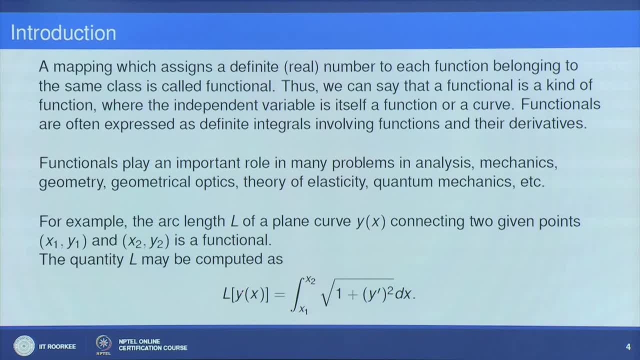 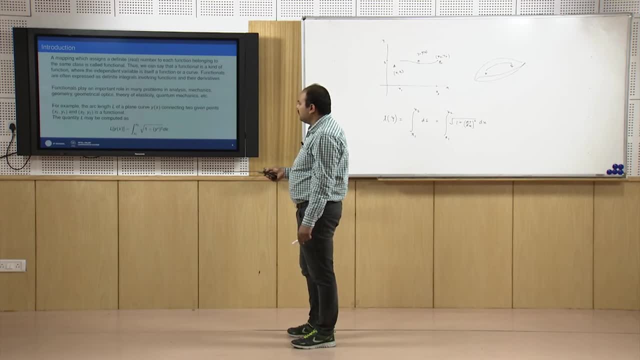 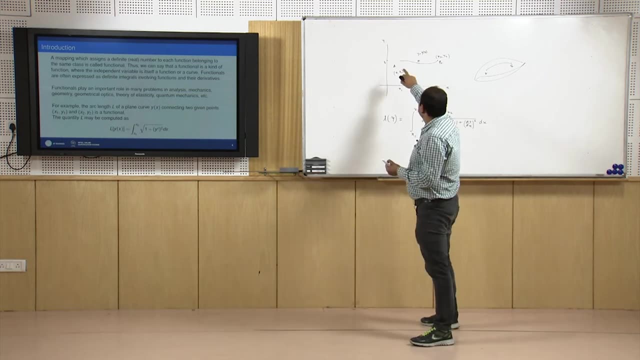 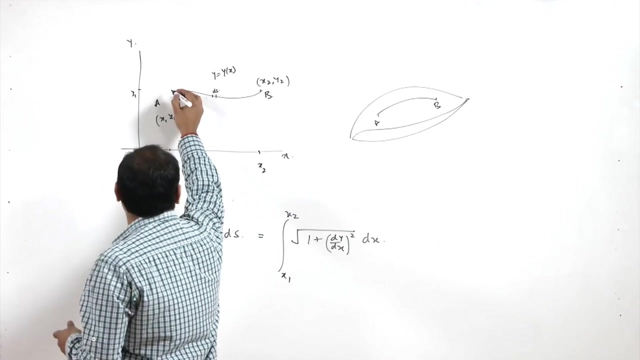 you use one function, you will have a one value of this infinite integral. If you use another function- y, x- then we have another value corresponding to that function. or you can say that, given one curve, there is a different length. If you use another curve, then we have a different length. So if we can use this, then this is y, this is y1.. 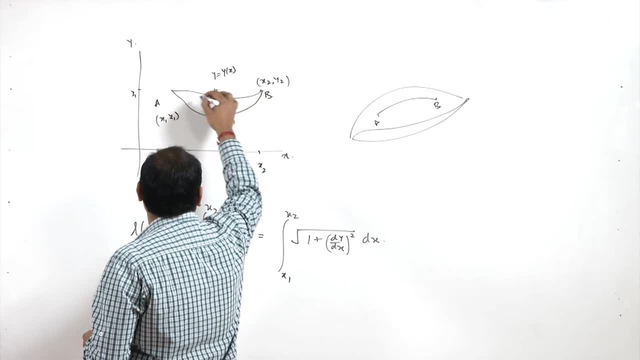 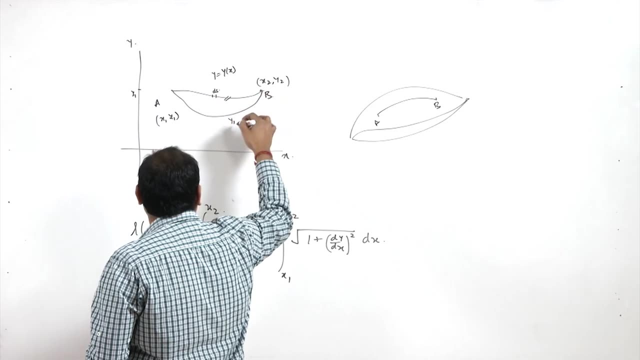 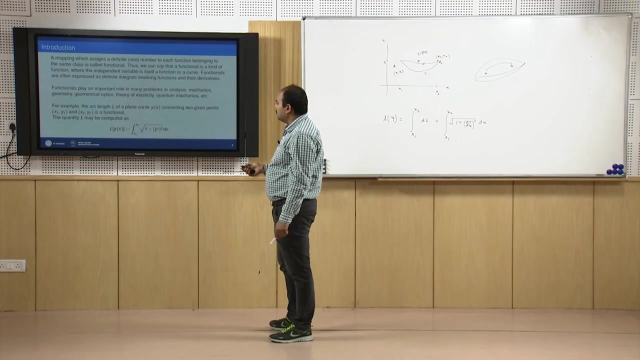 So we can say: here we have a value, or you can say length of the curve connecting through this curve, and we have another length if we use this y1 as a curve. So we can say that this L? y is a function of your variable y, which is a function of x also. So we can say that this 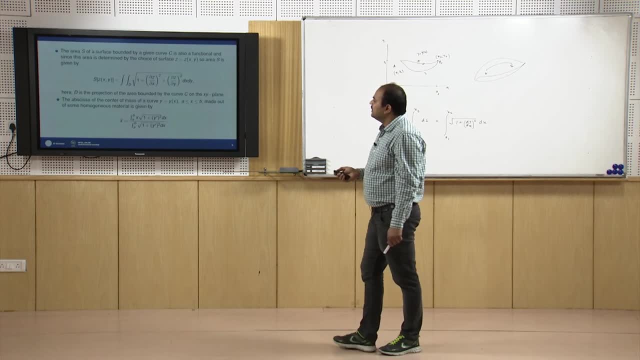 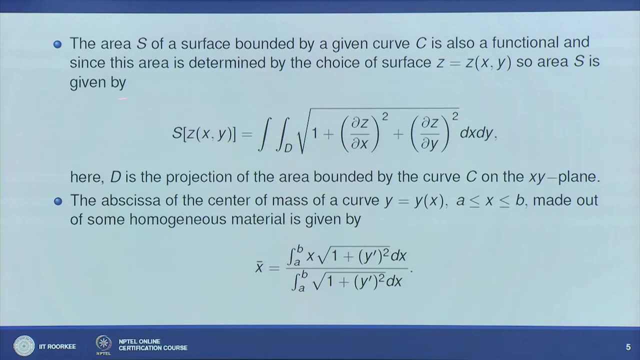 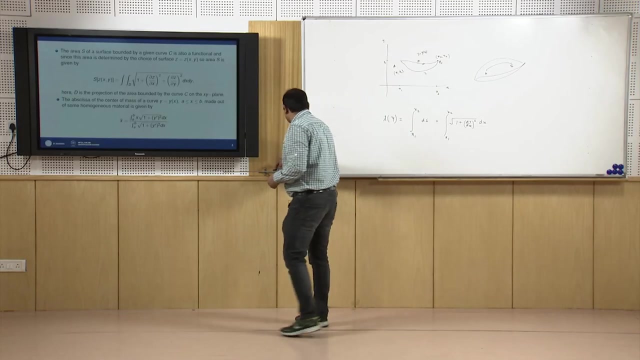 is a functional. Similarly, the area S of a surface bounded by a given curve is also a functional. and since this area is determined by the choice of the surface, So we have a, say curve C, So let us say that we have a curve C, So this is say the, this is the curve. 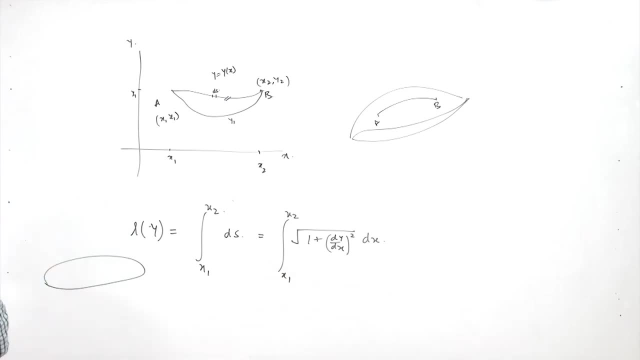 Now, here, this curve is bounded, So we have a surface, So we can say: we have a surface like this. We may have a surface like this and any you can consider like that. So we have a surface like this. and this is, C is the curve which bound this surface in this. 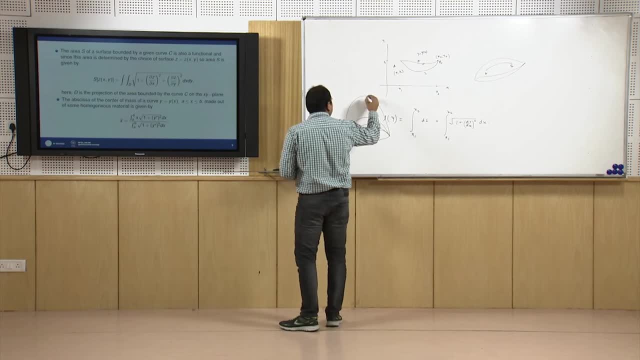 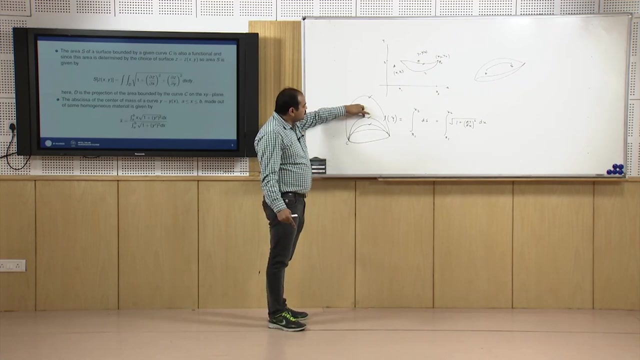 area. So here we can. we want to find out the surface area of these curves. So this is the surface area of these surfaces which are bounded by the curve C. Is it okay And we can say that if we choose this surface, then surface area is different, If we choose? 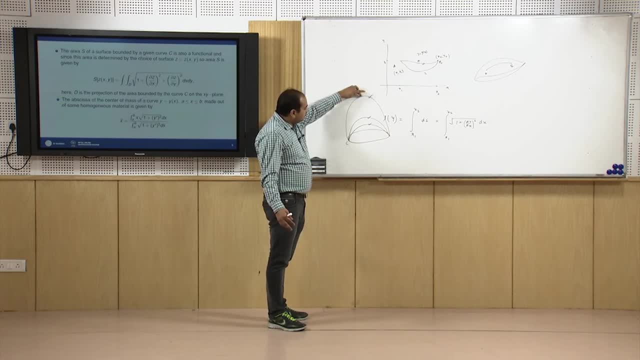 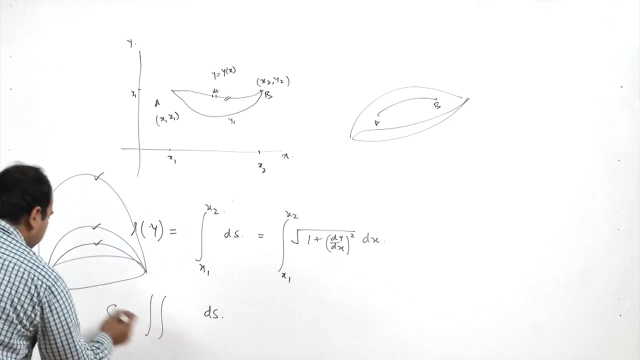 this surface, then the surface area is different. and similarly, whatever surface you choose, your surface area is quite different. So we can say that here your surface area S, which is given by say D of S over this region, we can call it say D dash, So we can find out the surface area based out this D of S. 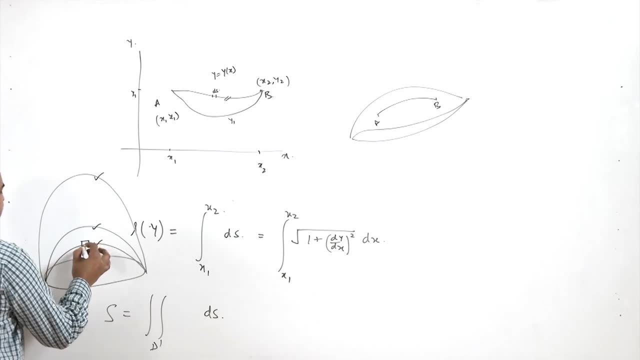 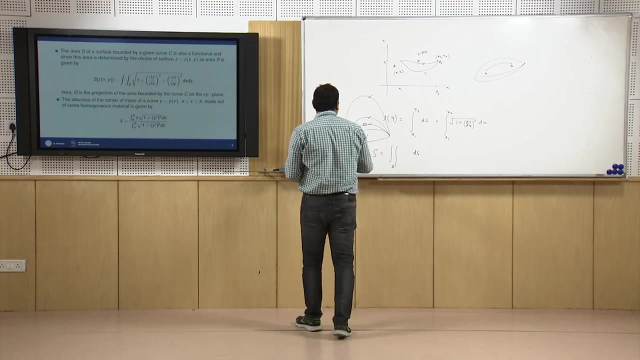 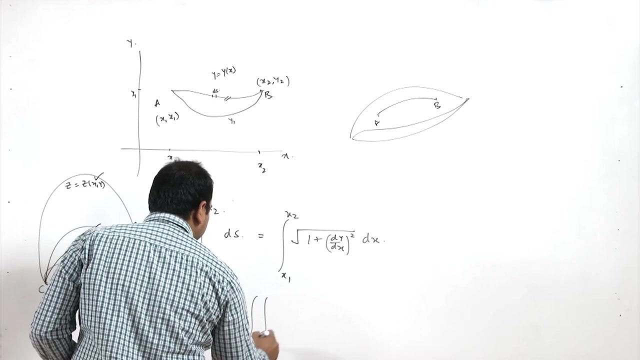 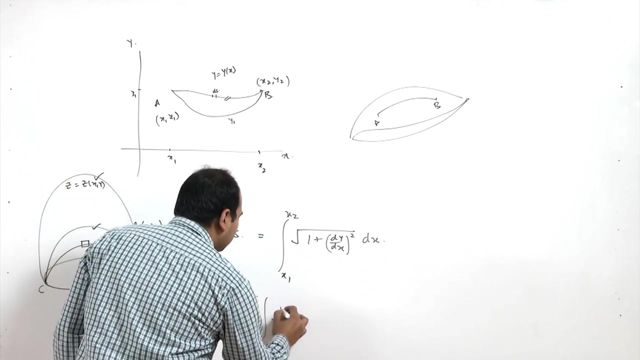 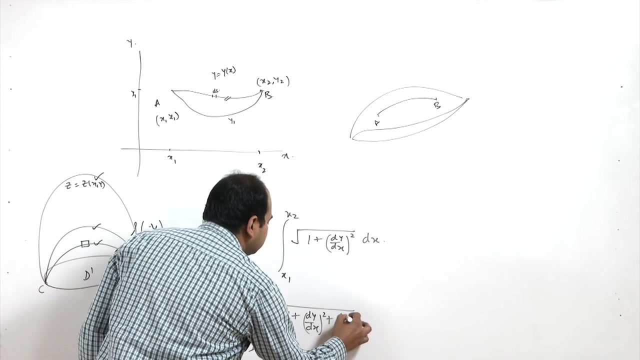 where D of S is the say surface patch on this surface D of S. So if I take, say, one surface z equal to Z of xy, and then this can be written as double integral over D, and this is this surface area element and can be written as 1 plus y. dash means d, y by d of x, whole square plus d, z by d of. 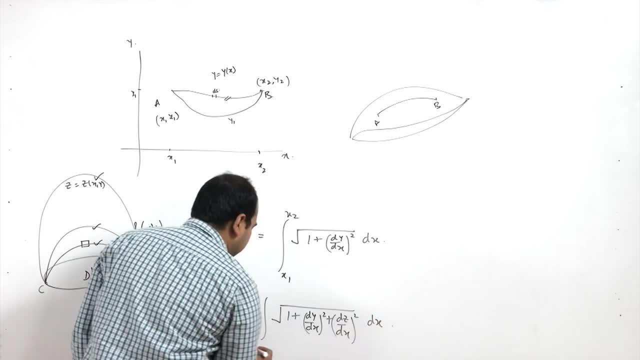 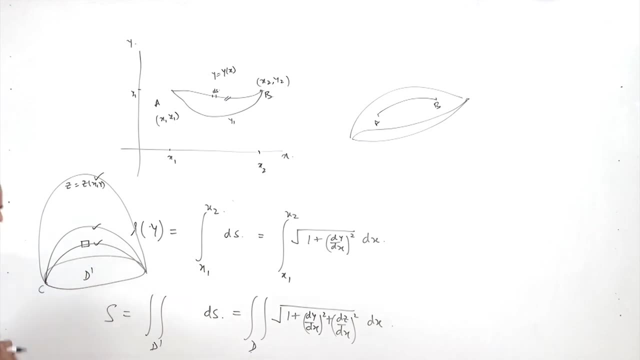 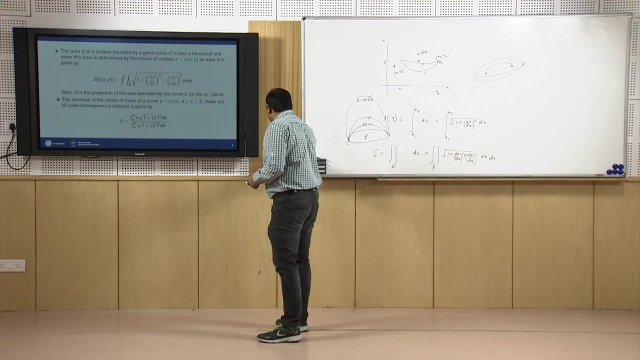 x whole square and d of x, and here d is the projection of this on x? y plane. So here d is denoted as the projection of your surface bounded by this c on the x? y plane. So sorry, here it is d x, d y. So here we can say that the area s of a surface bounded by a given 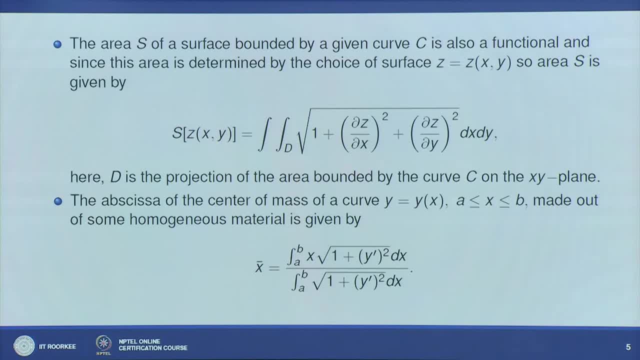 curve c is also a functional, because if we use a different surface, your surface area is different. and since this area is determined by the choice of surface, z, which is given as z of x, y, So area s is given by this. So here your functional related to surface. 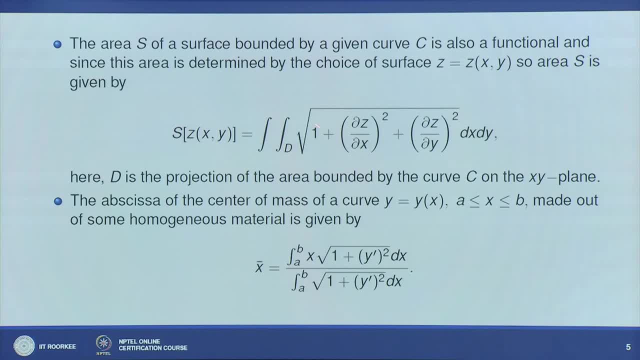 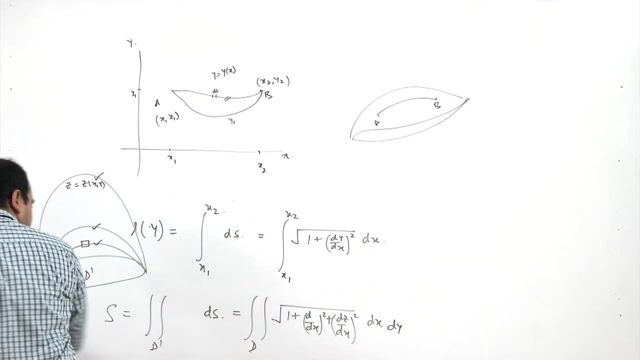 area is given by d Integral over d under root: 1 plus z dash square plus z y square, double z by double y square, d x to a y. So there is a small problem here it is, here it is, So there is. 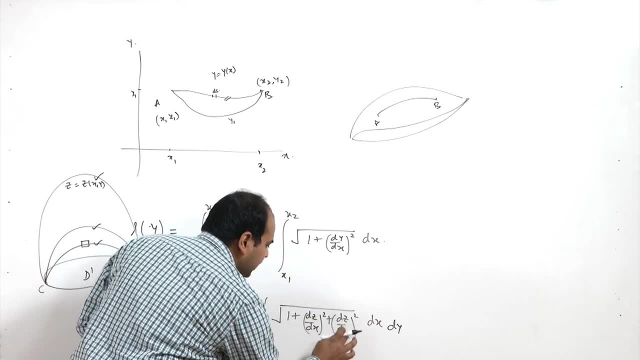 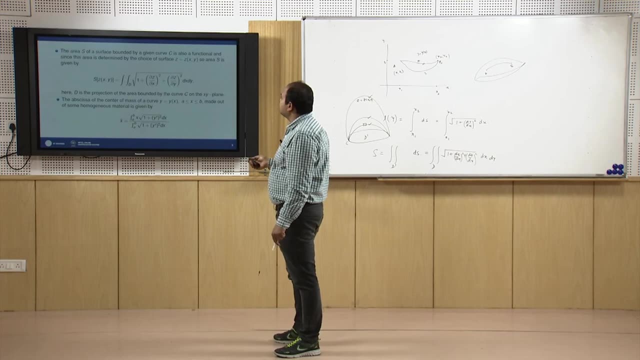 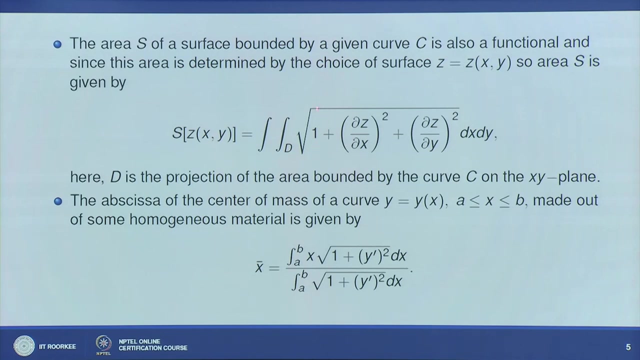 a wrong thing. So here it is d? z by d x, whole square, plus d z by d y, whole square. I am just correcting it. So here we can say that the surface area corresponding to the surface z, x, y is given by this double integral d, and this surface element can be written as: 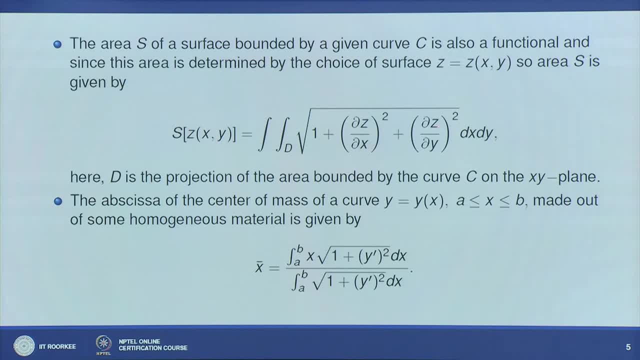 under root: 1 plus double z by double x, whole square, plus double z by double y, whole square. d, x, d, y, and here this d is the projection of the area bounded by the curve c on the x- y plane. So this is also an example of a functional 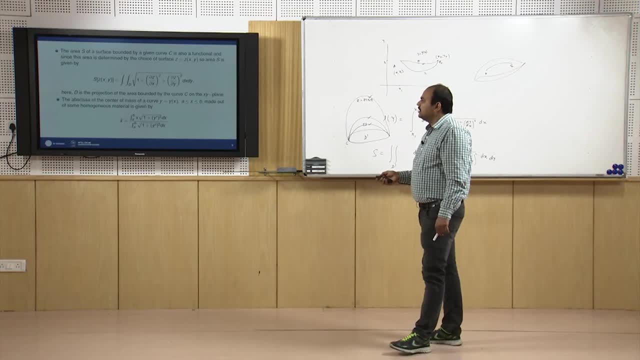 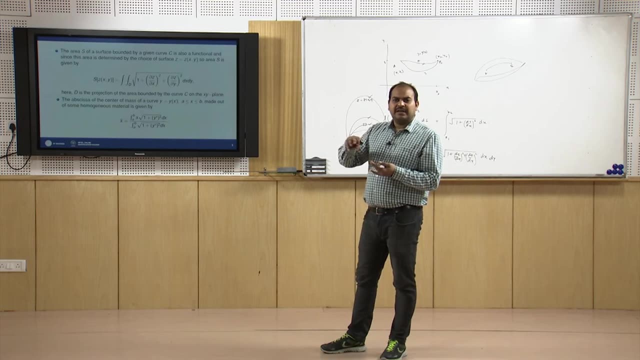 Now we may also define a functional in the sense of centre of mass. So if we represent that this function, y equal to y, x, is made of some kind of material, then we try to find out the centre of mass of this material. So this y of y, x will give you some kind of a. 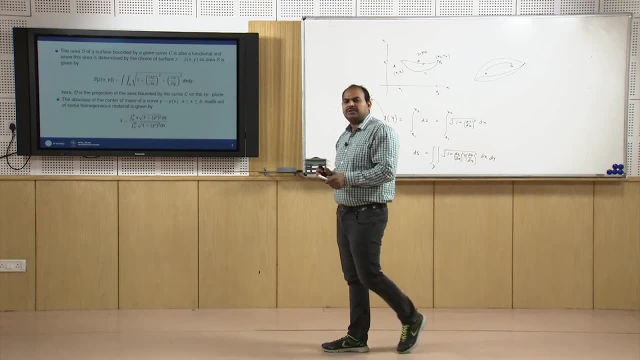 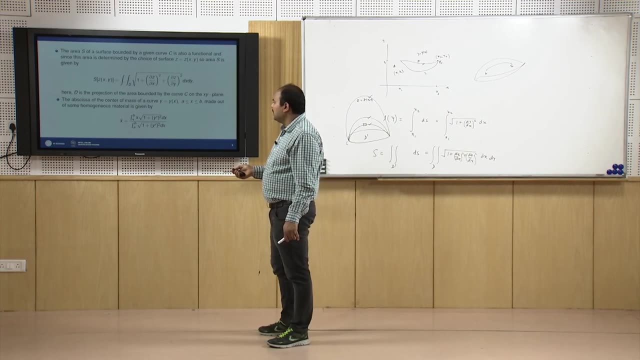 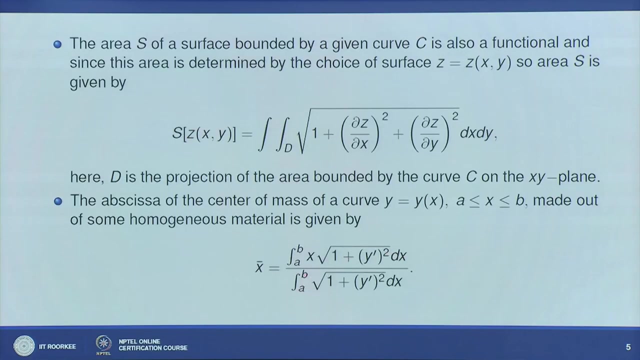 curve which is made by some material and we try to find out, say centre of mass here. So we can. we have already seen that this can be written as x bar equal to ratio of two functional a to b, x Under root 1 plus y dash square. d of x divided by a to b under root 1 plus y dash square. 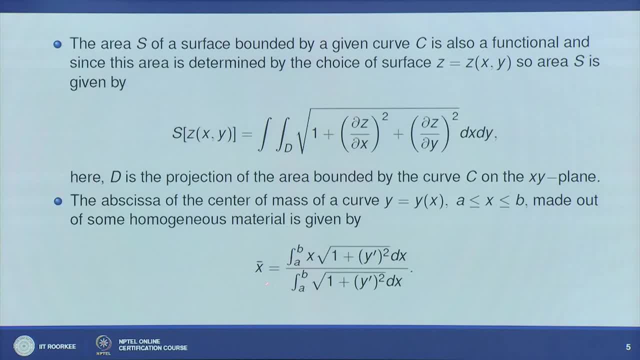 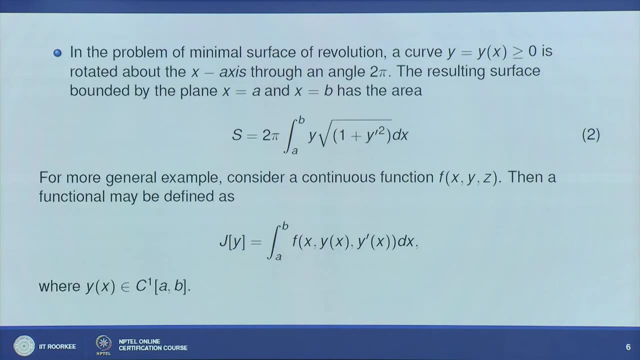 d of x. So this is the x component of the centre of mass. Similarly you can find out the y component of the centre of mass. So in that case your y bar is defined by you. simply replace by x by y. So this is also the functional. So it means that if you change, 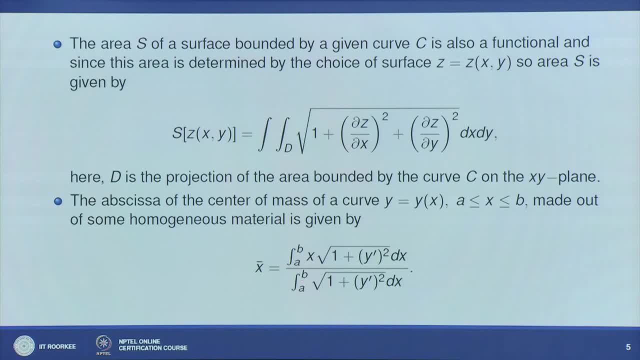 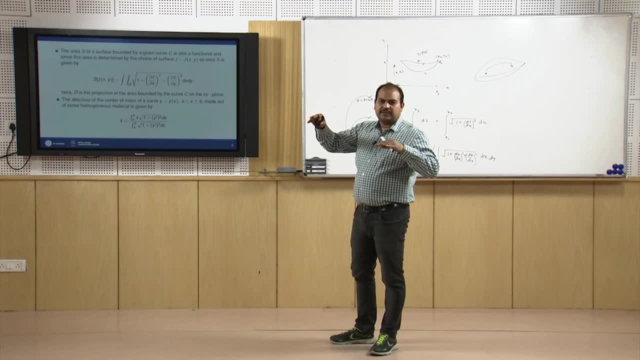 the y of x, Then your centre of mass is going to change. So it means that if you change this curve y, it means if you are changing the shape of the shape of the material shape of the say graph, then its centre of mass will also change. 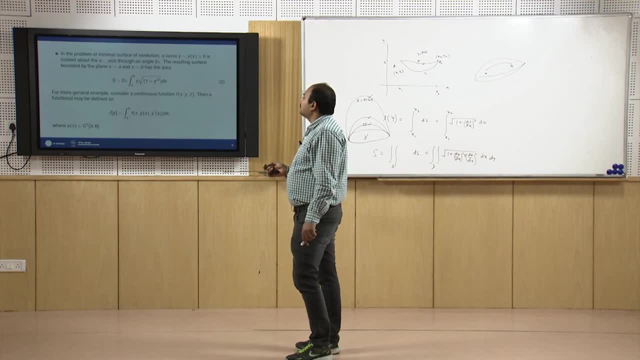 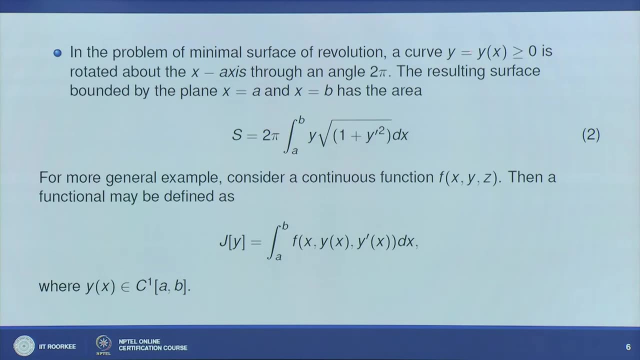 So next thing is the that the problem of minimal surface of revolution, this we have discussed- that if we have a curve, y equal to y, y, So this is the wave area of x, and is rotated about the x axis through an angle 2 pi, then 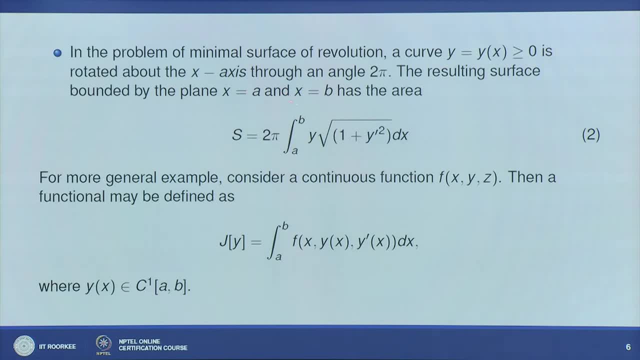 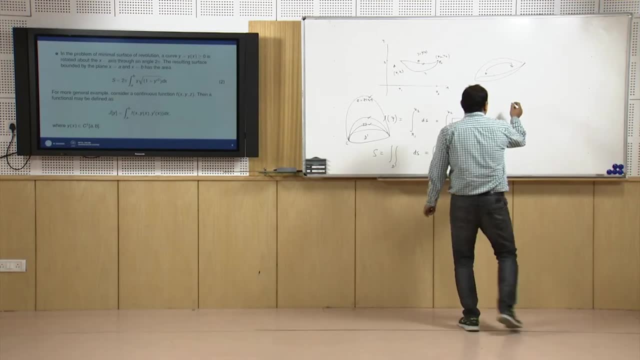 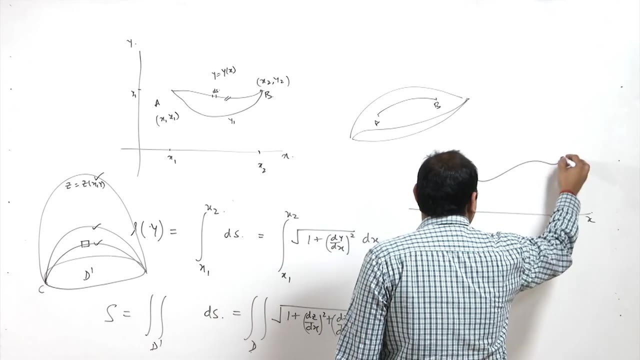 the resulting surface bounded by the plane, x equal to a and x equal to b has this area. So this we can write it like this, This we have in fact drawn, but let me write it here. So here we have: this is x, this is y and this is the graph: y equal to y of x and this is: 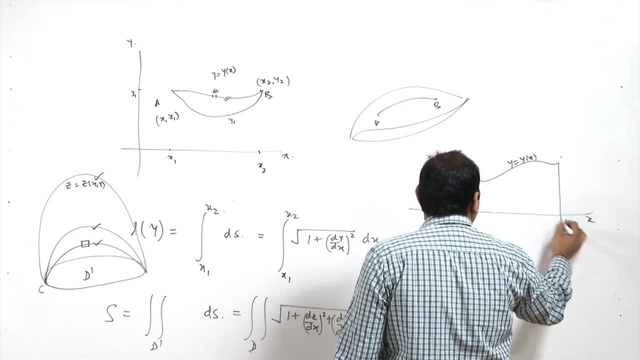 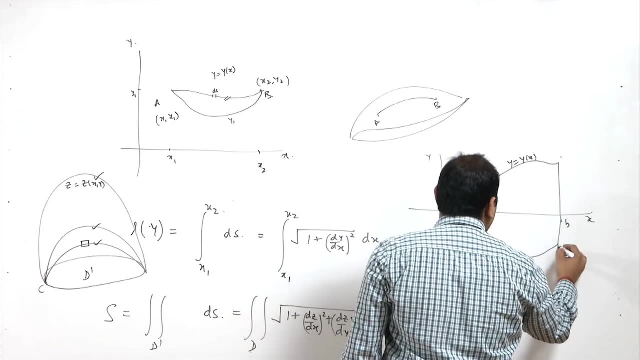 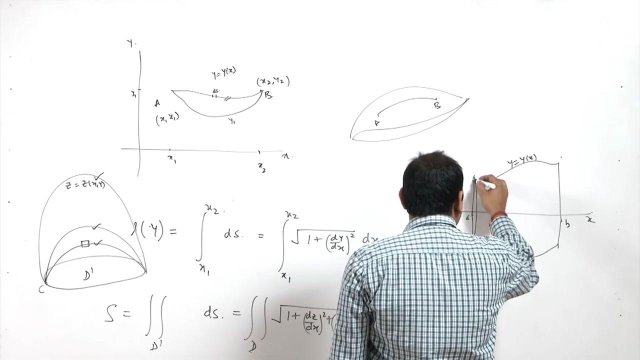 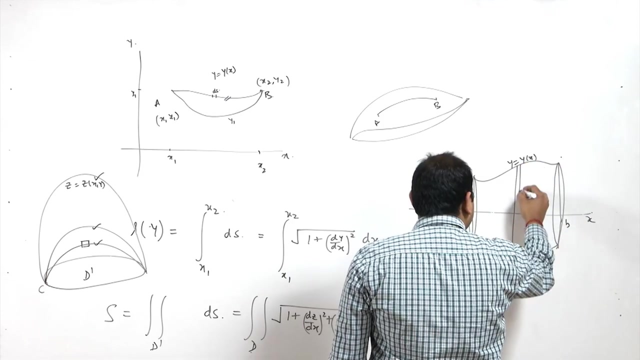 your a and this is b and this is rotated through x axis of say, ok, So it is this thing. So now we try to find out, say, surface area of this. So if you look at here this, we can patch it, this to entire shape, can. 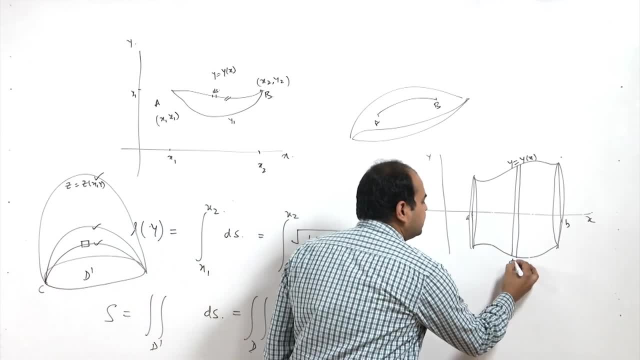 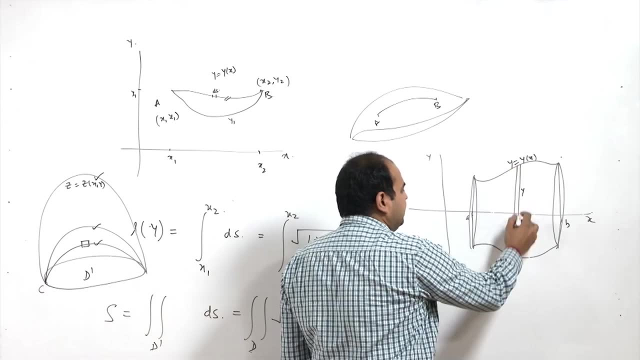 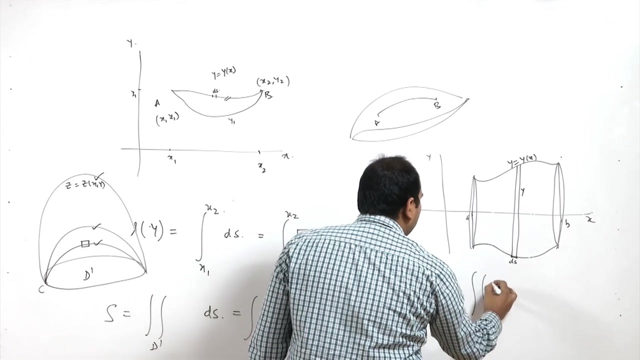 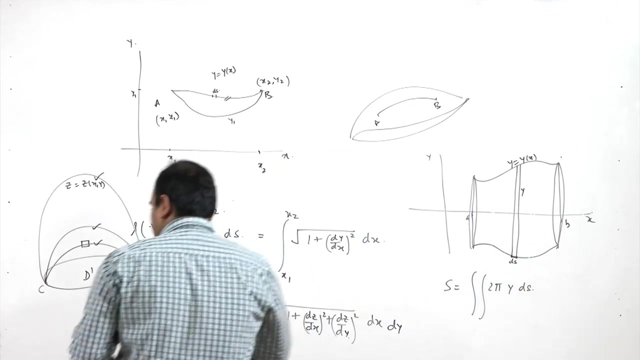 be truncated into these kind of patch and we can call this as patches. this is the surface patch, like D of s, and we can say that y is the say radius of this circular patch and you can say that the surface area is given by 2 pi, y and D of s. right Now here, since I am discussing only 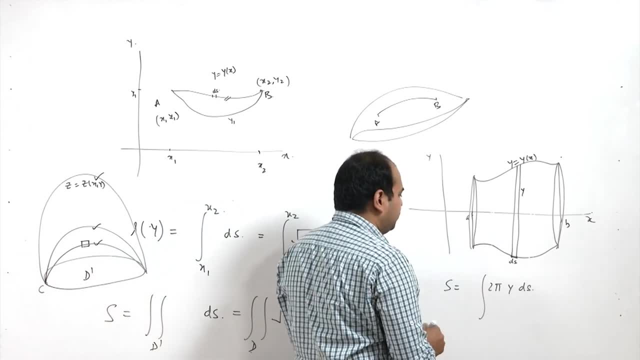 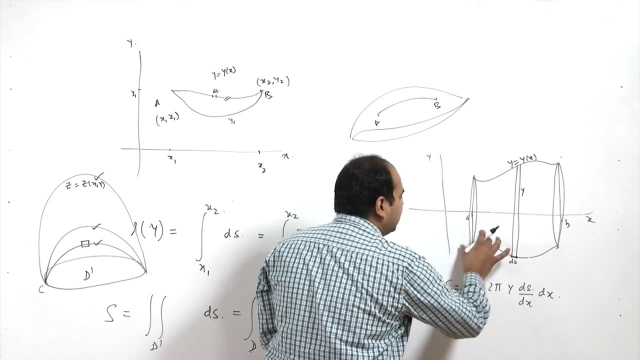 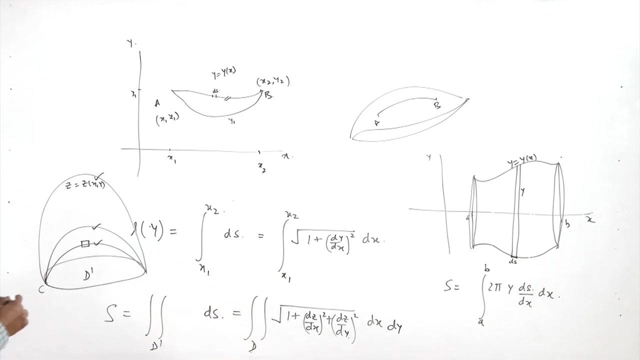 line integral. So we are considering only say single. So I, we can write it here: 2 pi y D of s, D of x, D of x. So and this is we are considering only between a to b, So we can write it a to b. So we can say that the surface area of this generated shape is given by 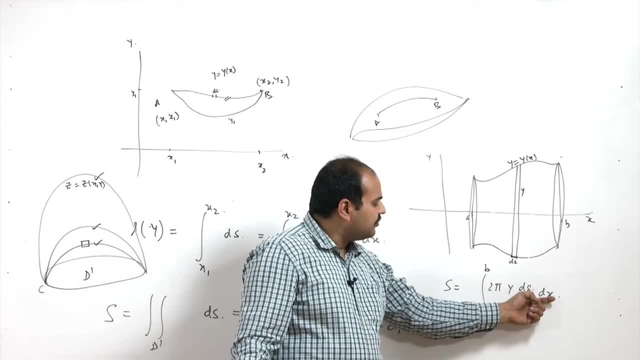 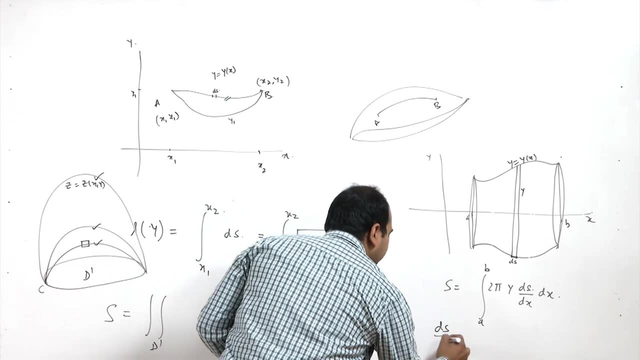 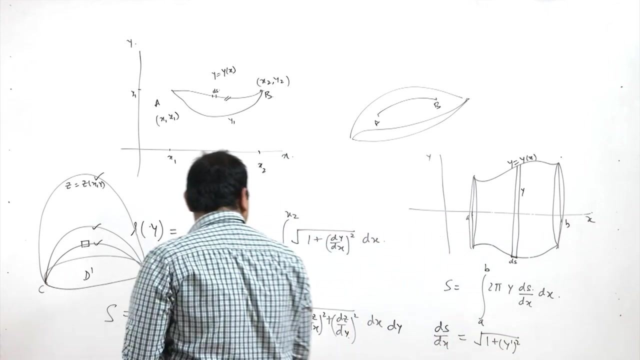 a to b, 2 pi y ds by dx, D of x. So you can find out: say ds of dx, as here you can write: ds by dx, x is equal to under root 1 plus y dash square. So here y dash represent dy by d of x. So 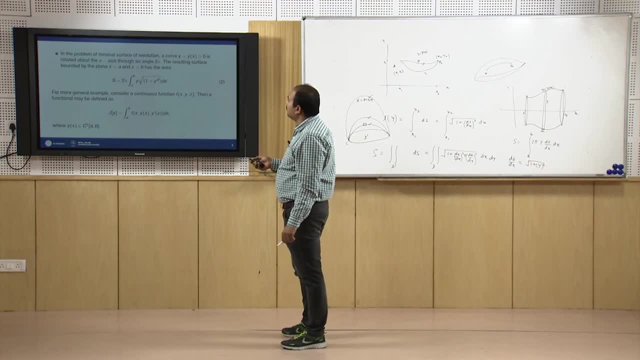 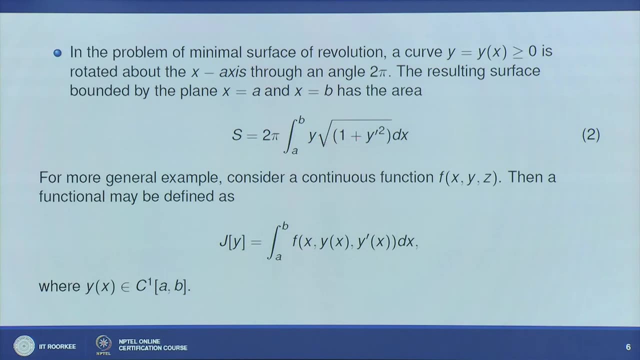 here you can say that the resulting surface bounded by the plane x equal to a and x equal to b, has this area s equal to 2, pi a to b, y under root 1 plus y. dash square d of x and we. so this is also one example of functional. 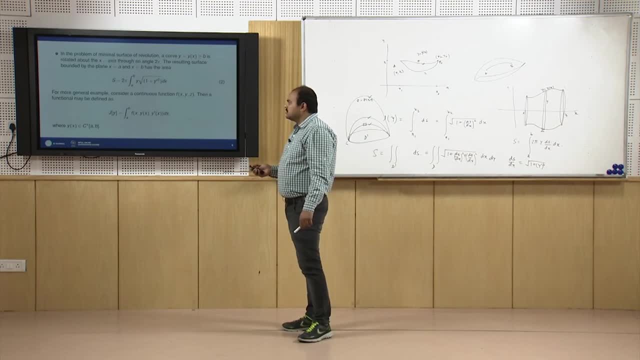 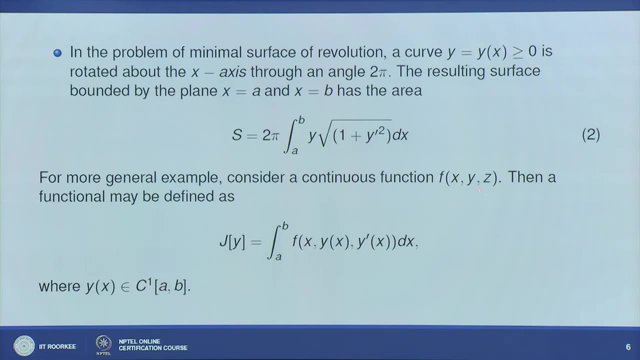 And if you look at in general, we can define, say, general example of functional as this: with the help of a continuous function f, which is continuous in terms of its arguments. so it means that function f is continuous with respect to x, y and z. then you can define functional. 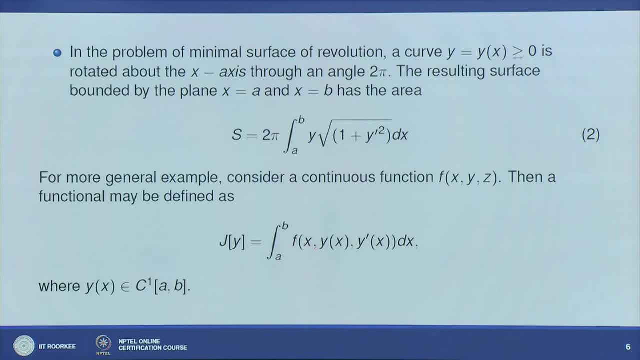 defined as this: j of y is equal to a to b, f of x, y of x, y dash x, d of x. So here, if you look at then, by taking a, A particular values of this f, you can say that this first problem, that is the length. 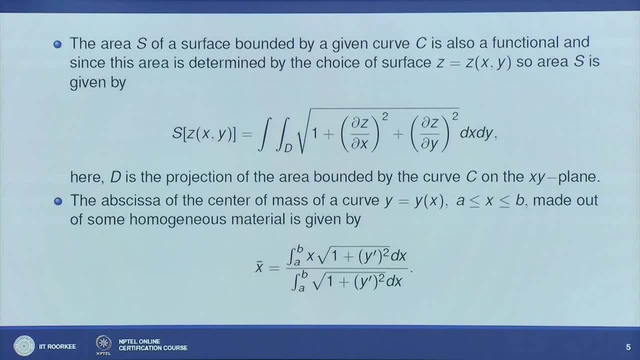 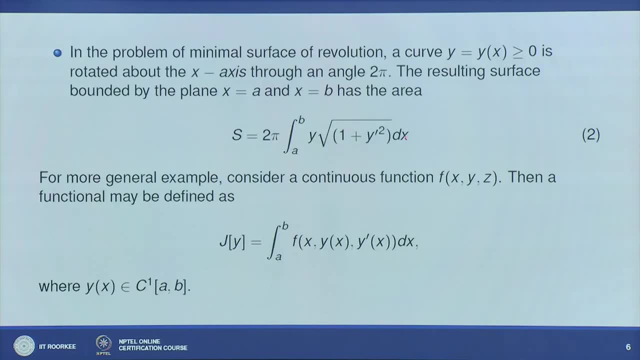 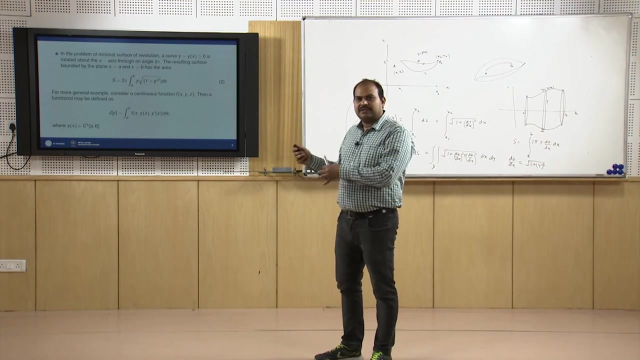 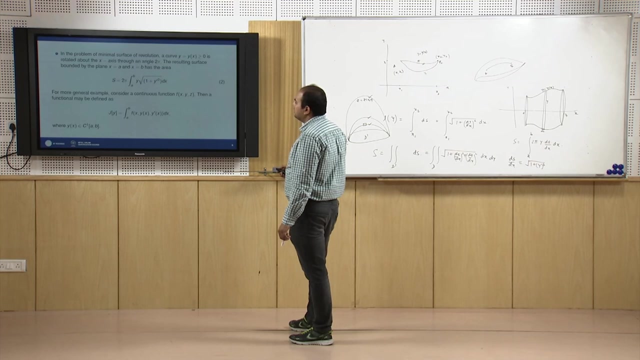 of the plane curve and the surface area and the this the area surface area is, also can be consider as a particular case of this. And here we may consider one more property, that is, these kind of functional, is a have having a localization property. what is localization property? that here we can truncate the region. 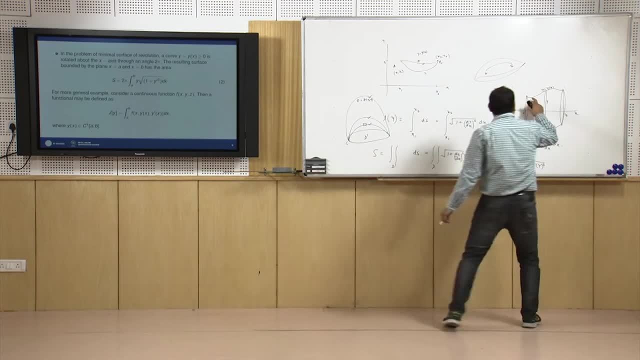 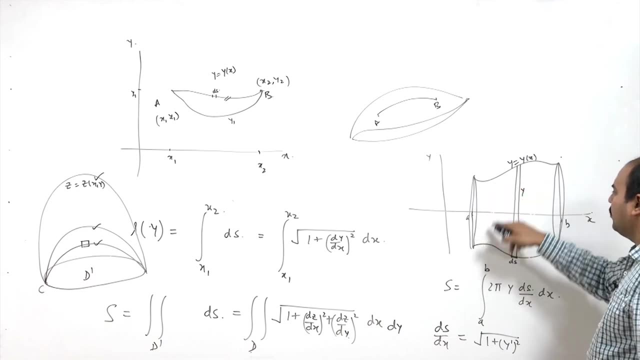 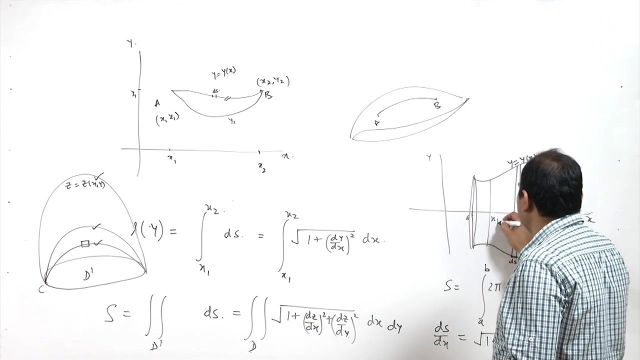 of y of x, for example, this particular problem here we can consider this y of y of x, and then we can truncate the region between a to b into smaller parts, And for each smaller part, for example, we have this a to say x 1, and then x 1 to x 2, and 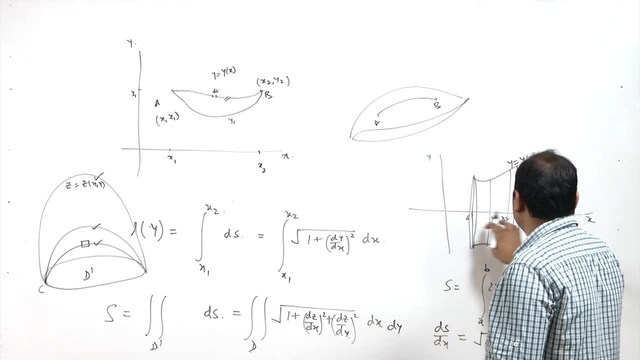 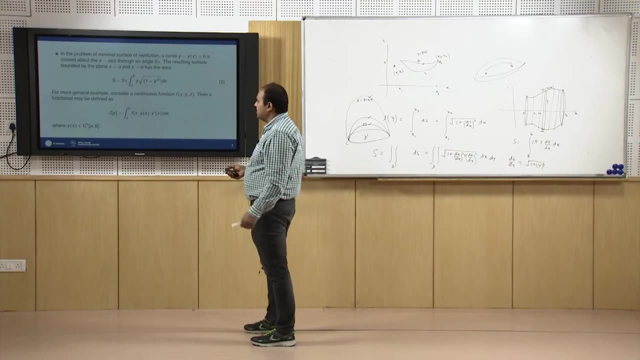 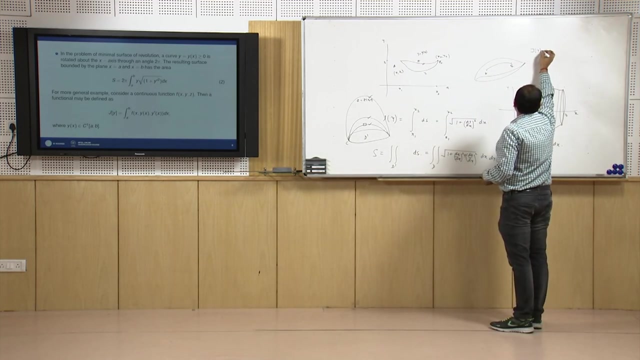 so on. So here we can divide this entire range a to b into several sub patches and we can find out, say, corresponding functional and find out the value of each functional. So it means that you can say that, for example, here we have j of y is equal to a to b and 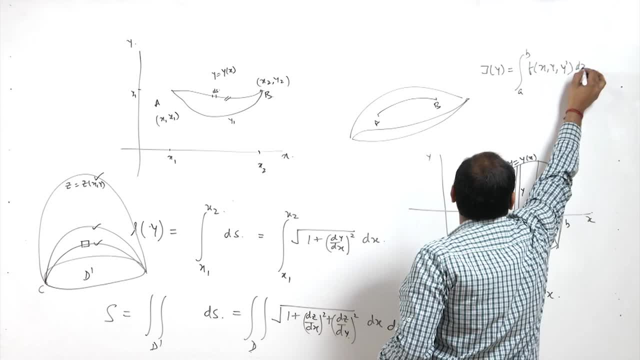 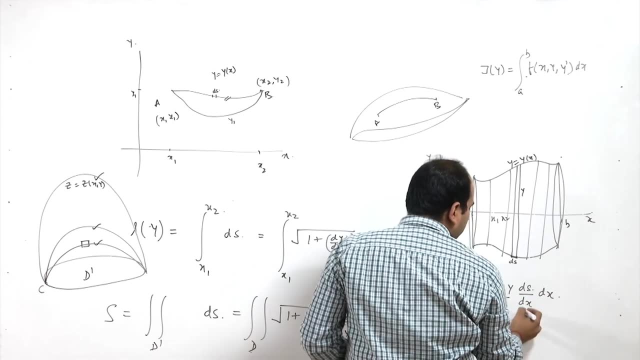 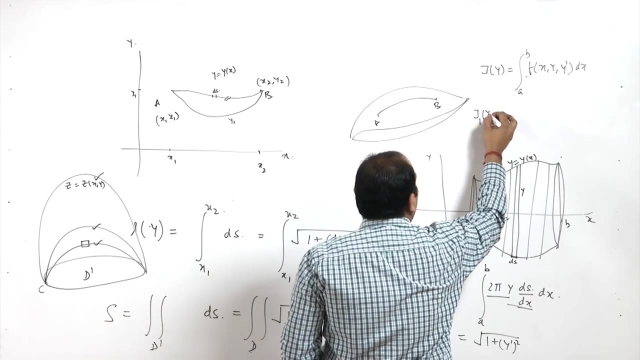 f of x y y dash d of x. So here in for this particular problem. your f x y y dash is given by 2.. 2 pi y d s, x, d s by d x. Now I am saying that if we want to write it, say j, 1, y, what. 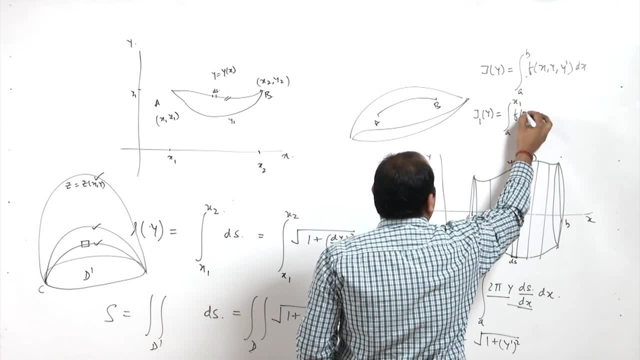 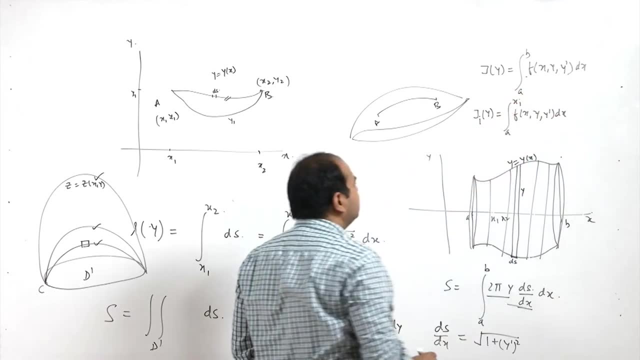 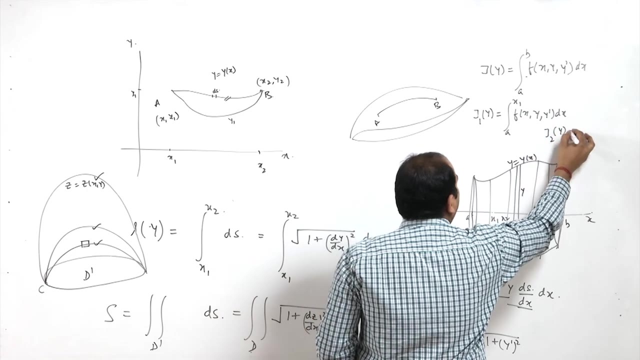 is j 1 y. here you write it a to x 1 and f of x, y, y dash d of x. So you can say that j i is nothing but this, sorry. so j 1 is between a to x 1. similarly you can define j 2, y is: 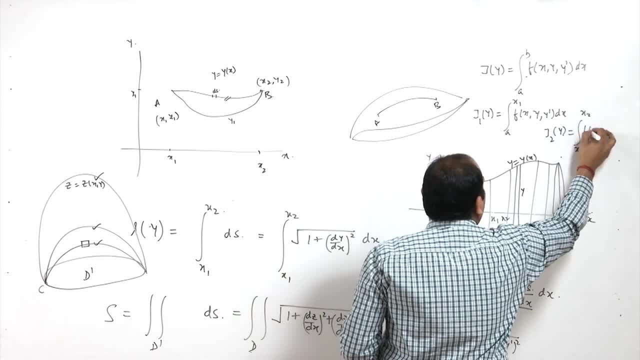 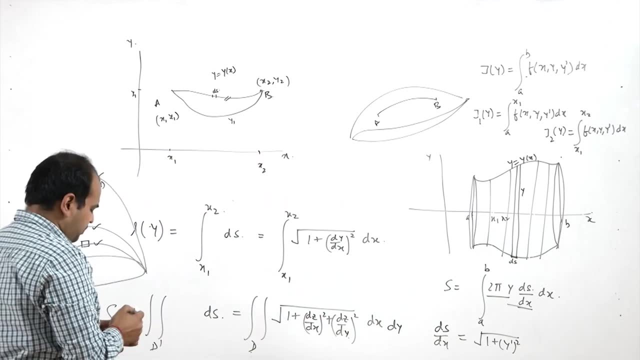 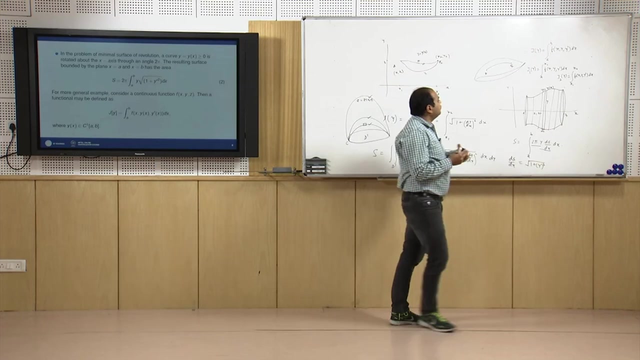 equal to your x 1 to x 2.. f of x, y, y, dash d of x. So similarly, you can find out patches, find out, say, functional defined in these sub patches and then if you sum all these values, then you will get the values defined by this original linear functional, original functional defined by j, y, equal to 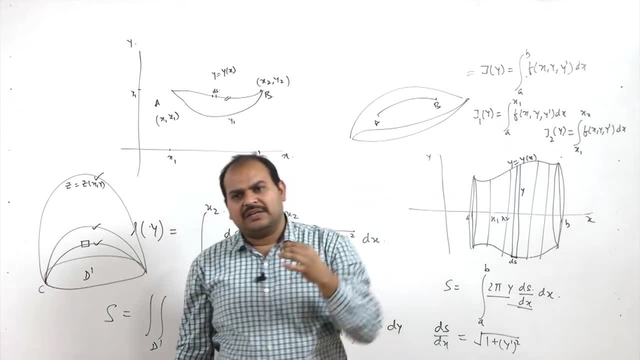 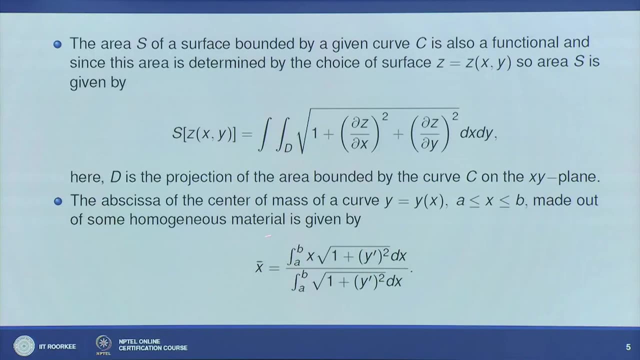 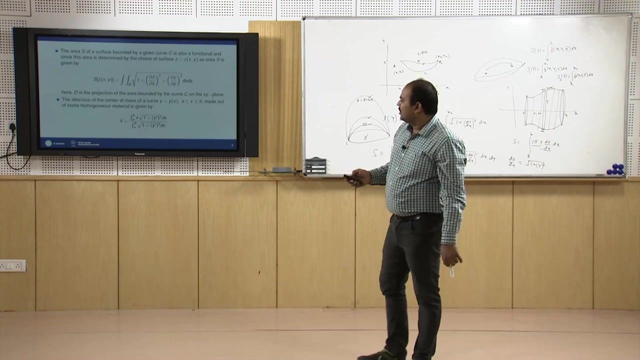 a to b, f, x, y, y, dash d of x. So we can say that this has a localization property. but if we consider this part, the functional defined here, this is not having this property. here we cannot do all these thing, So we call these kind of function as non-local functionals, and in calculus of variation we 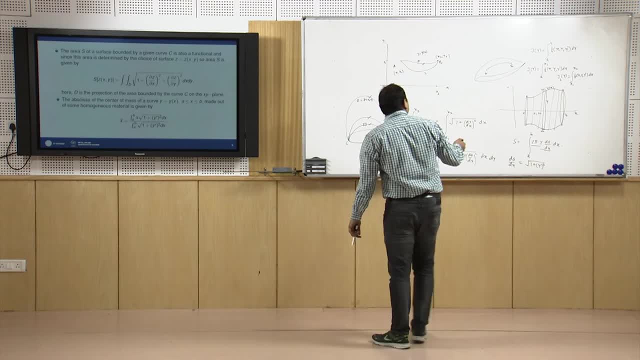 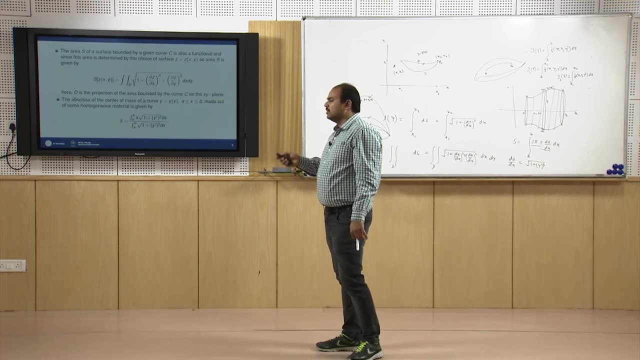 generally deal with the functional or with the localization property. So in calculus of variation we generally deal with local functional, ah, ah, ah, not this non-local functional. There are certain functions available, some methods available to deal these kind of problems. Therefore, for more general example, 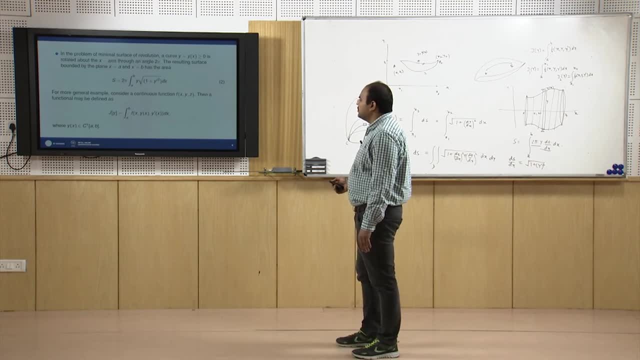 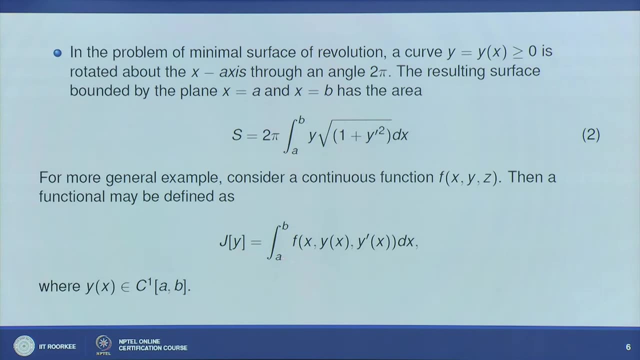 we can consider a continuous function- f, x, y, z- which is a continuous function with respect to its argument. then a function may be defined as: J of y, equal to a to b, f of x, y of x, y, dash, x, d of x, and here, by taking a particular examples of f, you can consider that the problem. 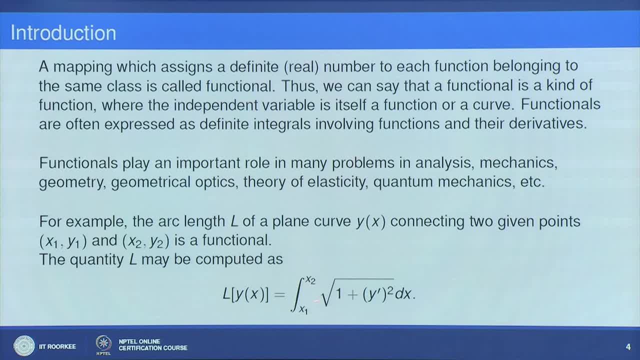 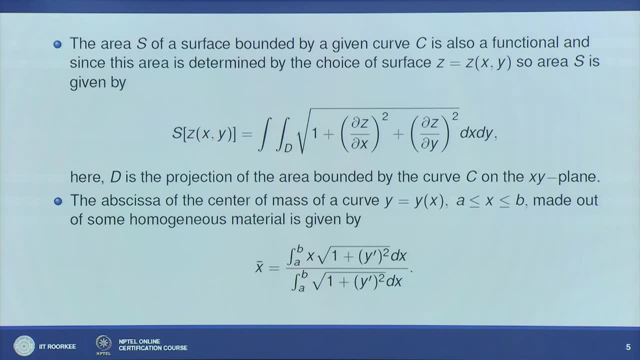 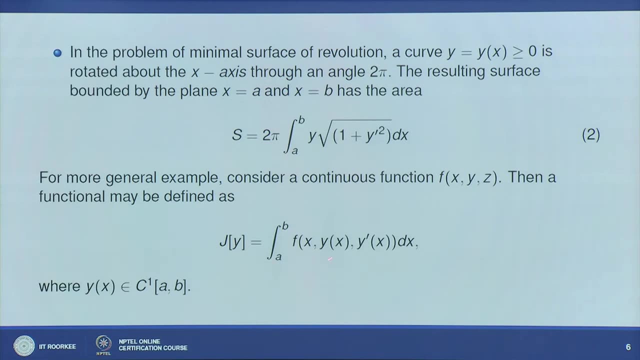 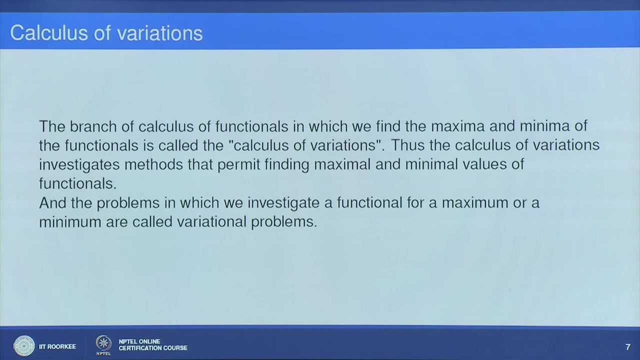 this problem, which is the arc length of a plane curve and the surface area of a surface bounded by, say, a given curve, C, and the problem of minimal surface of revolution given by this equation number 2, is a particular case of this right. So here, summarizing all this, we can say that the calculus of variation is a branch. 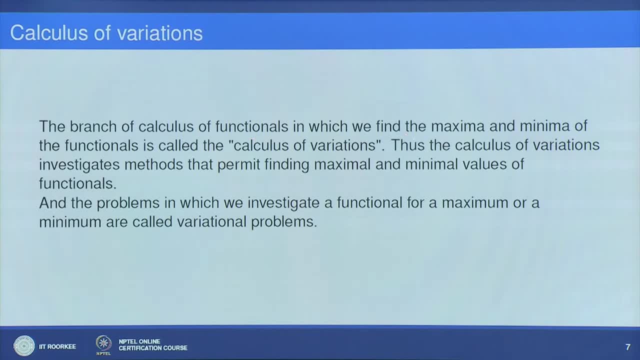 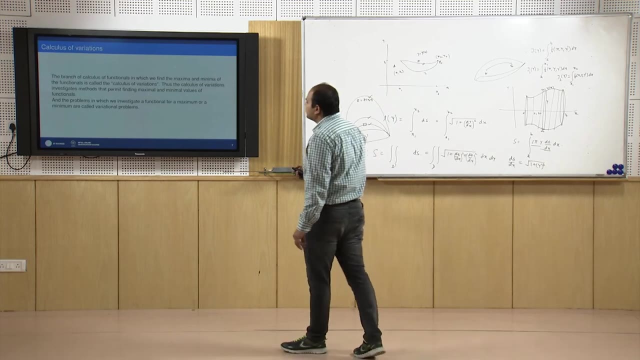 of calculus of functionals in which we find the maxima and minima of the functionals, And we can say that there is the calculus of variation. in this branch we discuss the methods that permits finding maximal and minimal values of functions and the problems in which. 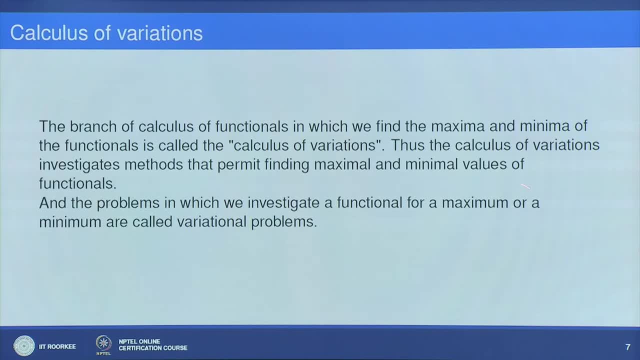 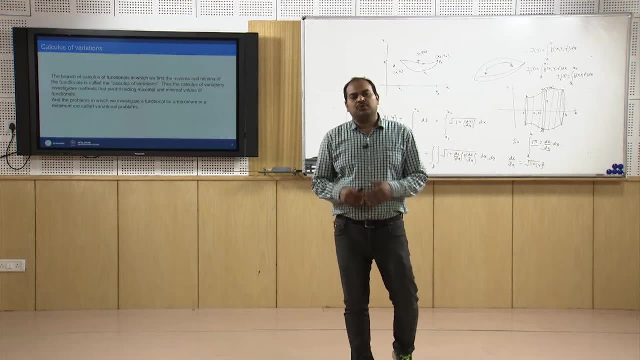 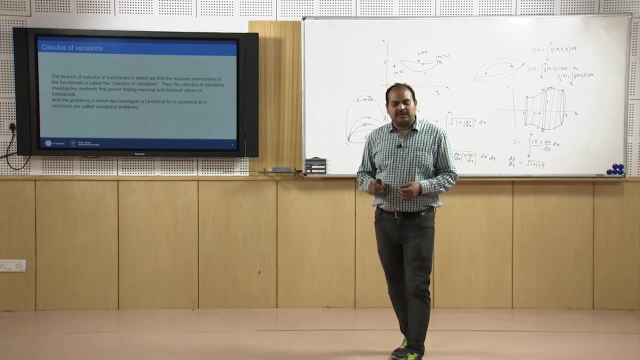 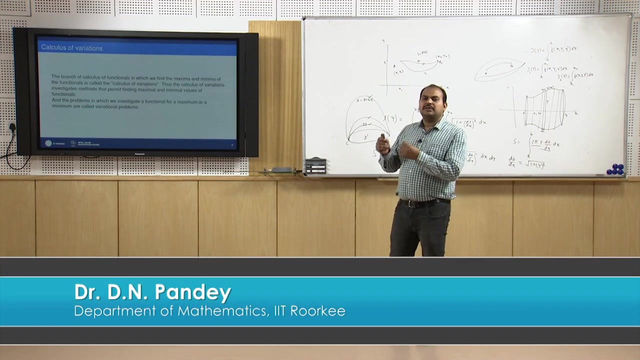 we investigate a functional for a maximum or a minimum, or called variational problems. In fact, there are certain principal rules in mechanics and physics that can be related to functional, that can be related as the maximizing or minimizing some kind of functional in that process.